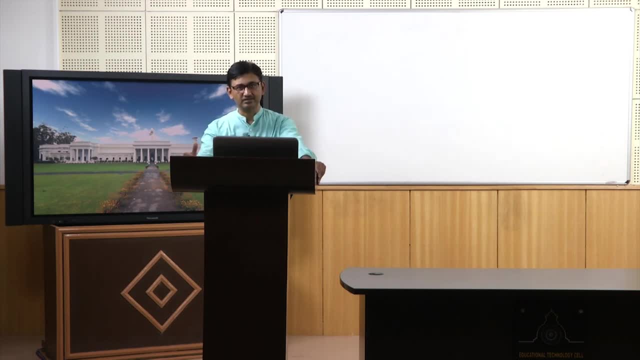 powers in this phase. transformation process will always be a stable system. if it is Gibbs, free energy is small, so for having a smaller. 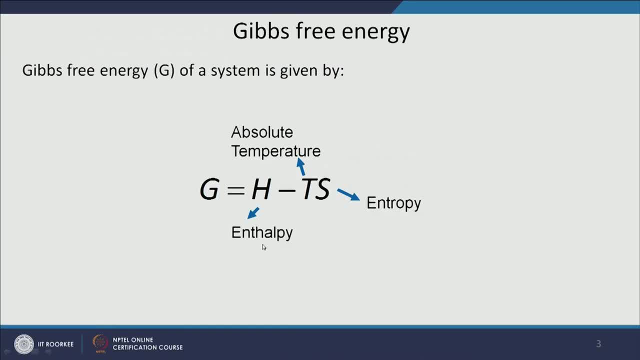 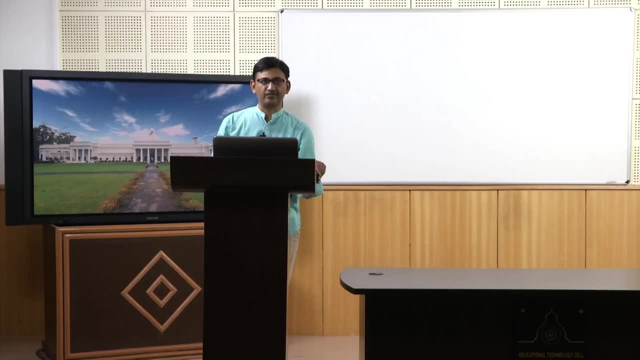 Gibbs free energy, either enthalpy has to be low or entropy has to be more, because there is a negative term in front of entropy. now, to understand this concept of Gibbs free energy, I have I like this particular slide which I made, that what how I can explain this three. 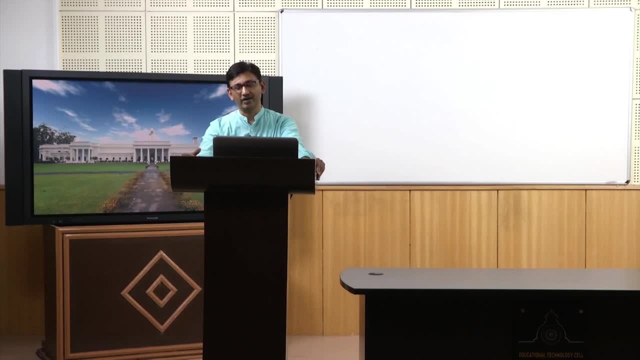 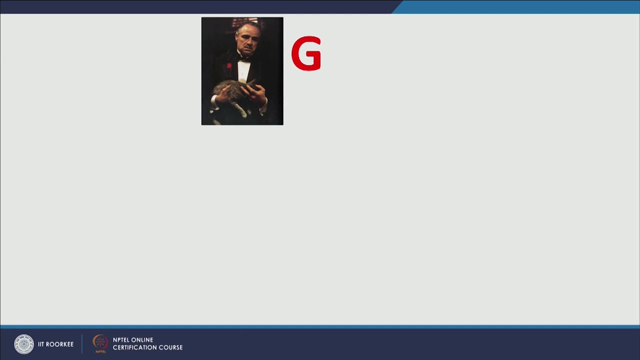 terms of Gibbs, free energy, enthalpy and entropy. and I take this analogy of one very popular novel called Godfather. there was a movie, also big, very successful movie, on that and I say that the Godfather, Which is G, which also relates with the Godfather, he is the G, the Godfather, and this is a very 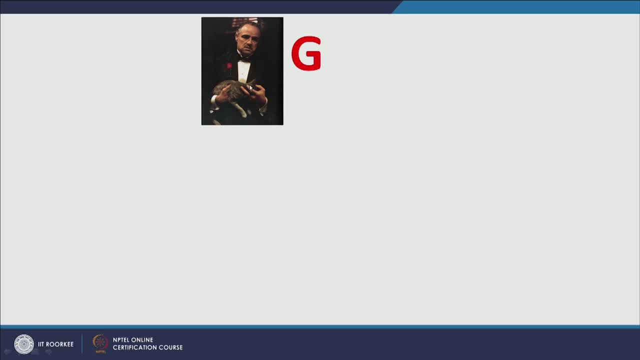 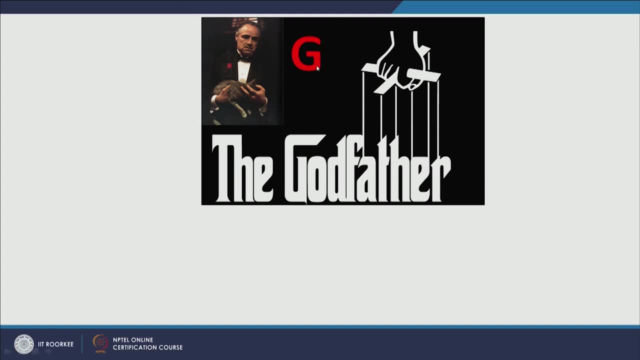 famous actor who portrayed this particular role in the movie and he is kind of playing with the system. and to help him in playing with the system there are to agents. so one agent is which is in there term- in Italian it is called capo regime, and these two are enthalpy and another one is entropy. so these 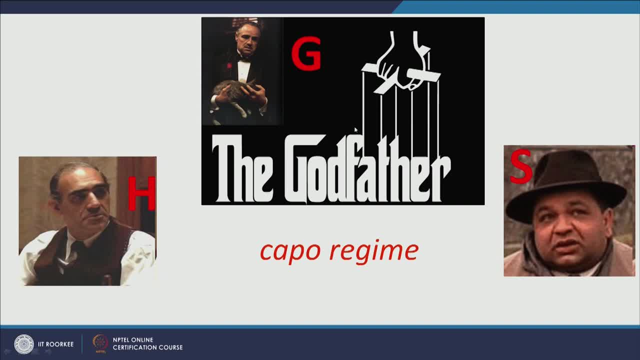 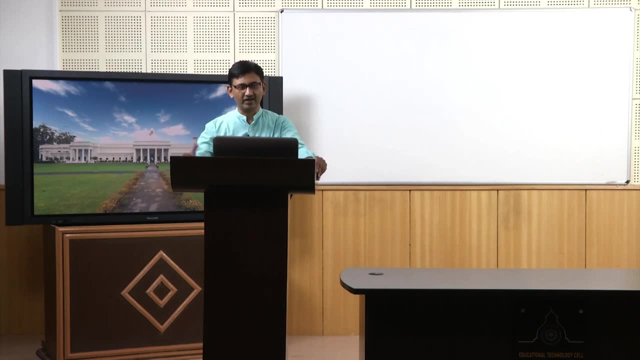 two are helping him, the godfather, to play with the system. and there, instead of we. usually we say, when any industry is there or any firm is there, that their motive is to make profit. here we can say, in terms of gifts, free energy, that their motive is to bring down the losses. 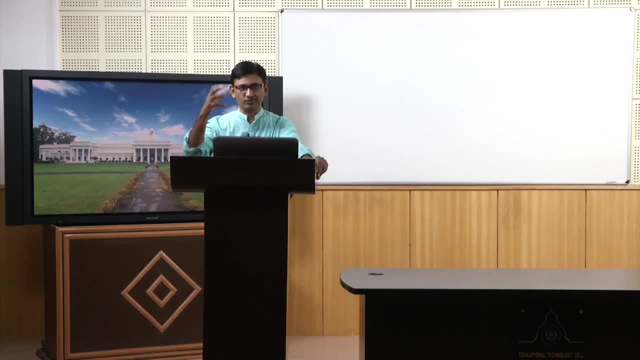 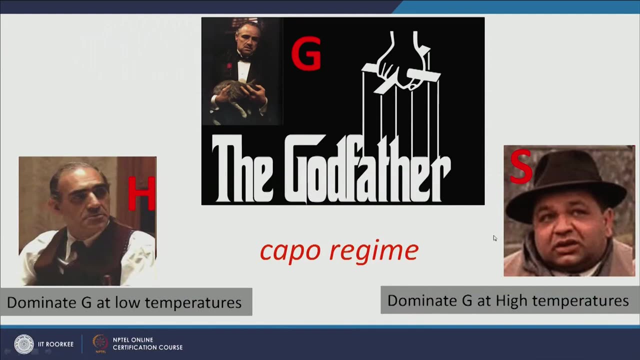 so these two guys will help to bring down the G, so they have fewer losses. and both of these guys, these two his main guys, they have a region of where they operate. so, for example, enthalpy will be dominating the free energy At low temperature. so at low temperature enthalpy term is more important. that means 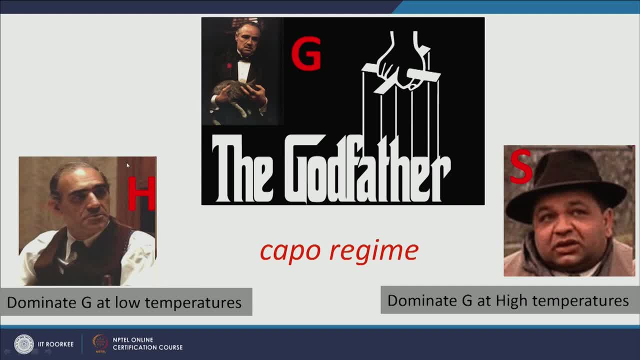 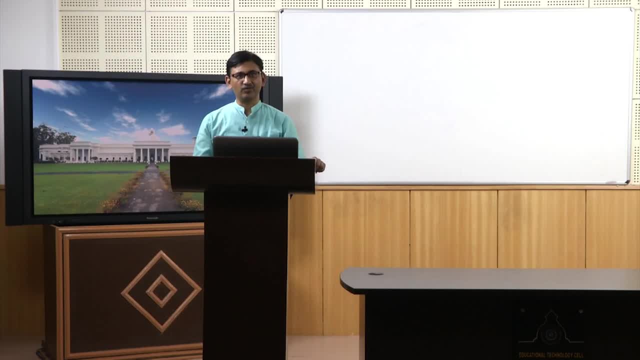 it is his region of where he will play or where he will operate, because, you can understand, a godfather has large number of people who are helping him. they he want to give them separate area so that they do not interact with each other and the entropy will dominate. 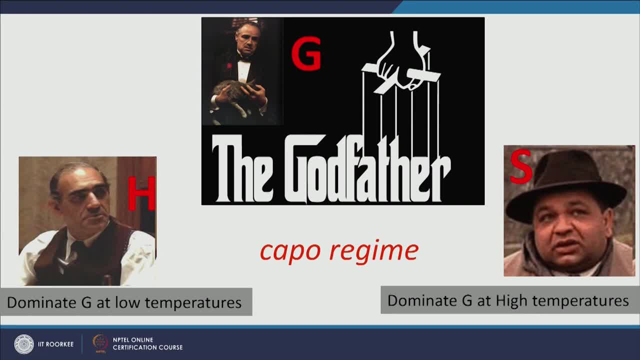 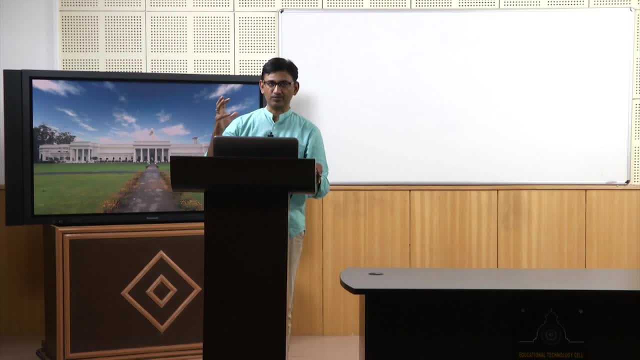 the free energy at high temperatures. So they have their own area. So they have their own area, So high temperature. whenever you come with a system which is at high temperatures, you always remember that entropy should be the term which is going to dominate the free energy. 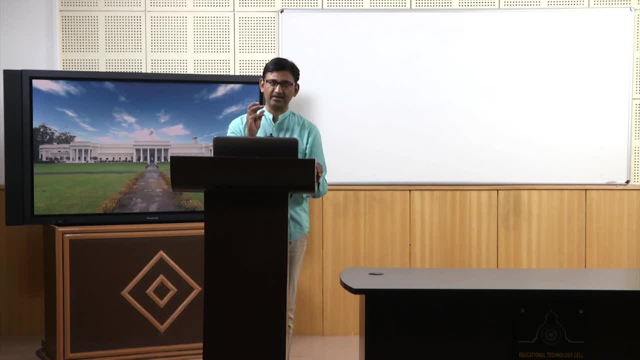 and when you are at a low temperature you should always remember that enthalpy is the term which is going to dominate the free energy. I am not explaining here the enthalpy and entropy parts because I assume in your mechanical engineering course it will be done in the thermodynamics course, so I am not going into. 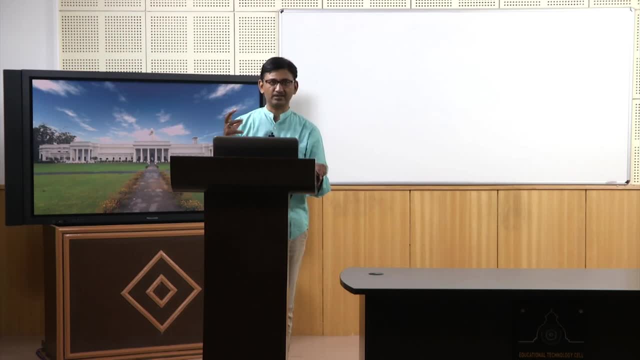 details of enthalpy and entropy, but there is a term called free energy, which depends on enthalpy and entropy. that is what we are interested in, and this free energy is also going to define whether my system is going to be in equilibrium or not. 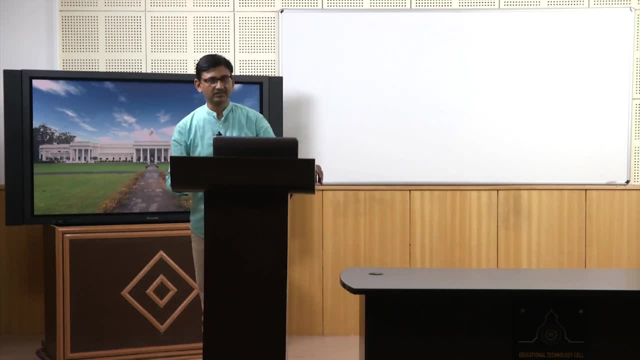 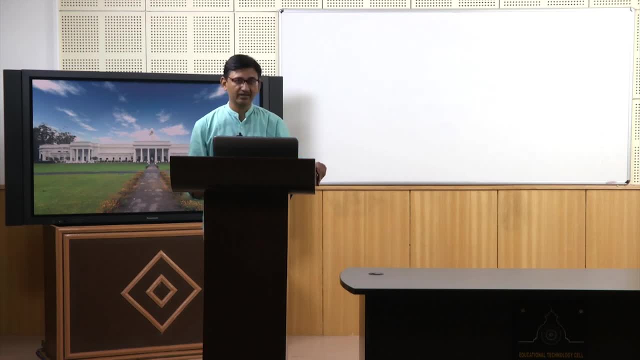 stable state. What do we mean by that? when I will say it is a most stable state, That it shows no desire to change at infinitum means it will not change. you keep that system for any length of time and it is not going to change, then it is a stable. 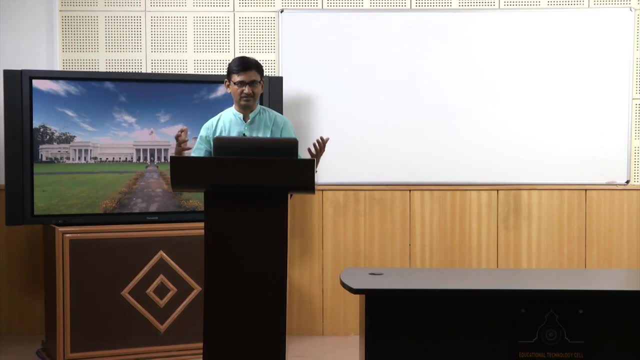 So you are a stable. when you do not want to change, do not want to change. if there is any instability, there has to be some change in the system. so the more stable state means I do not want to change, so at a constant temperature and 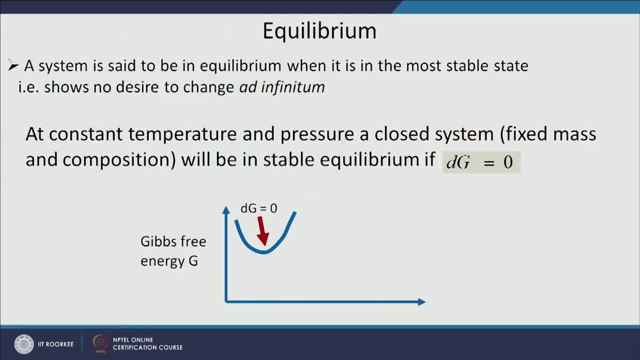 pressure in a closed system. closed system means it will have fixed mass and composition. so there is no change in mass and composition. there is no change in temperature and pressure. so different states. you can draw a Gibbs free energy curve as shown in the slide. you can. 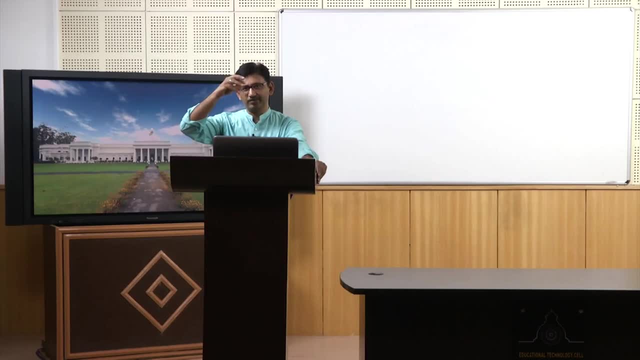 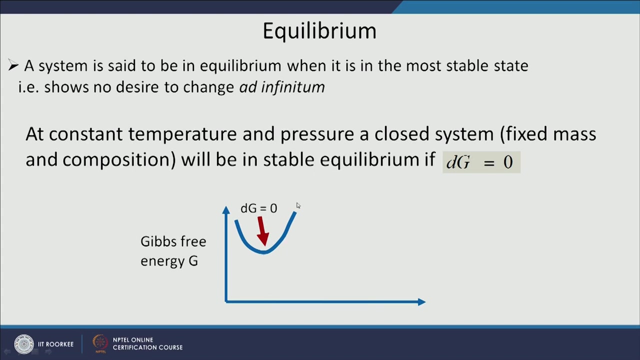 see that Gibbs free energy calculate. basically, you keep changing the states, different state, what will be the Gibbs free energy? you will get a curve, something like this: so stable state for this particular system which is showing a Gibbs free energy curve like this is when it has a minimal state. 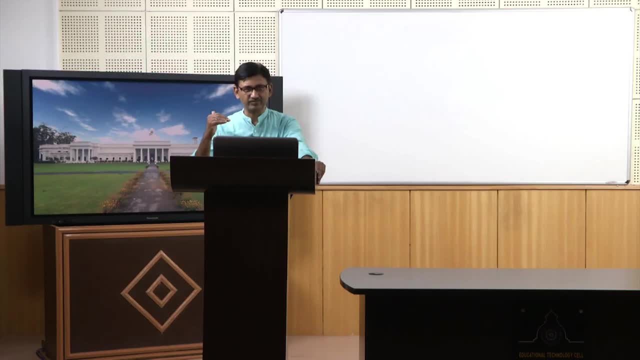 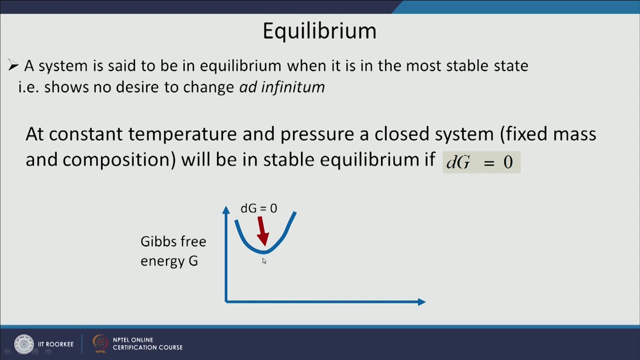 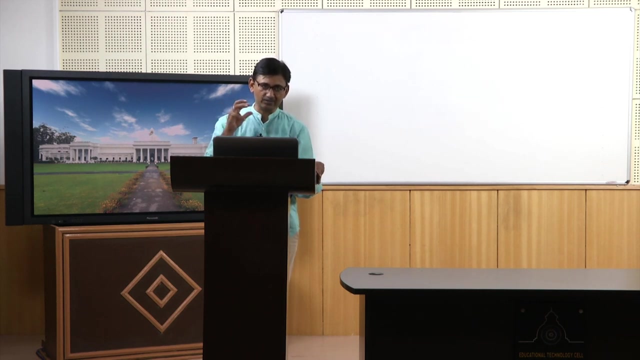 So, when it is going to be minimum, when the slope of this particular curve- if I draw a slope at different points, the slope of this curve will be 0, that means the DG is going to be 0, so when you have this particular condition, that is the condition for a stable. 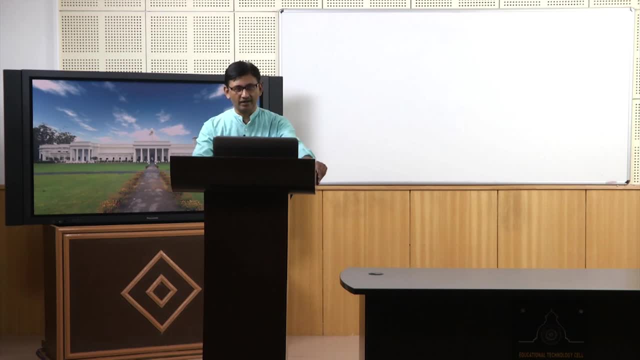 equilibrium for any system In this state. it is not going to change. it is most stable. so DG is equal to 0 should be the condition, but now you will see that there are more scenarios in which this condition will be met, and all conditions, all those condition are not the stable condition. so 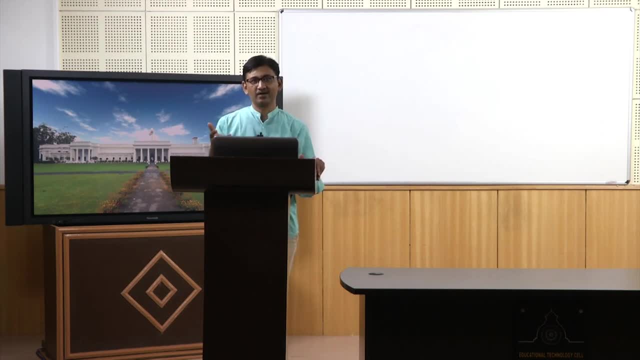 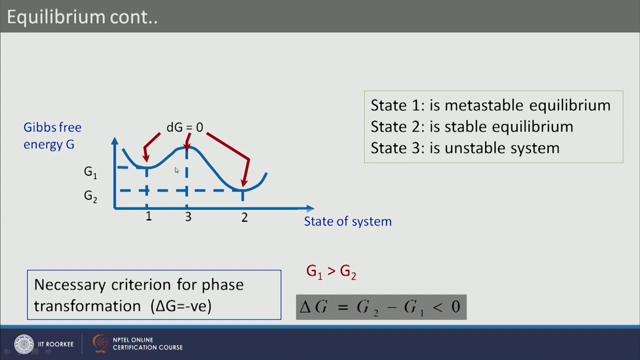 we have to kind of define more that. what do we mean by this? So DG is equal to a state in which the exact location your station is the base, condition in which station is the base, alright, Now the state that is the slope, in which the slope will be zero. 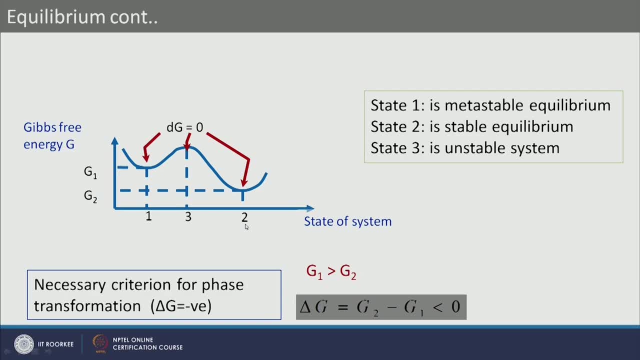 So we have to include the slope and slope information because all the commitments for each location will be change. who, okay? So we are calling it. state 1, stay 3, 0 at each location When you draw a slope, there is only zero condition at that position, which is we are calling. 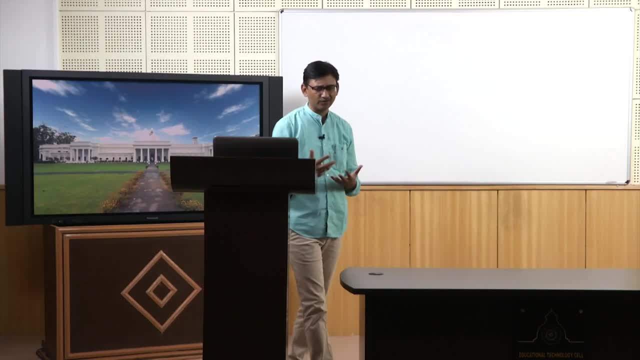 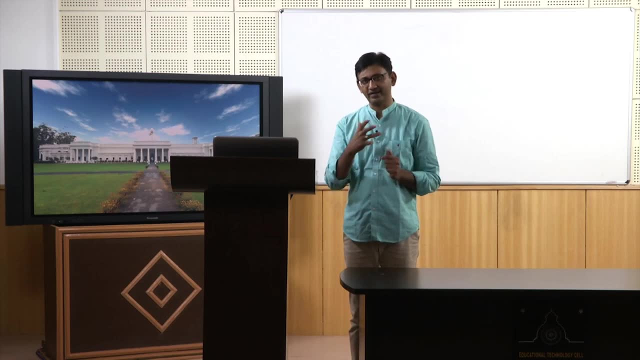 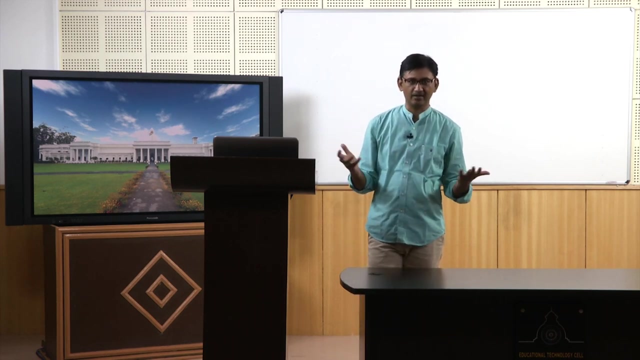 condition 2, okay, now you can argue that why this? different states will be there for a system. okay, so to explain that, I will take an example of carbon. okay, for example, carbon exist in free as a free carbon, okay, or it exist as graphite, or it exist as diamond. 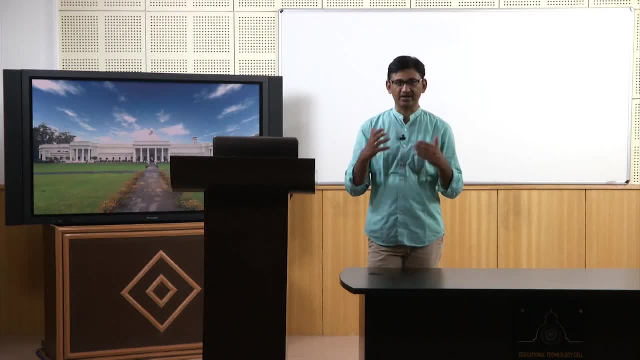 okay, so it has 3 allotromops. okay, 3 different crystal structures are there. okay, and this, the diamond, is not the stable state for carbon at normal temperature and pressure condition. so if I put diamond right now here, okay, that is not a stable condition for diamond. 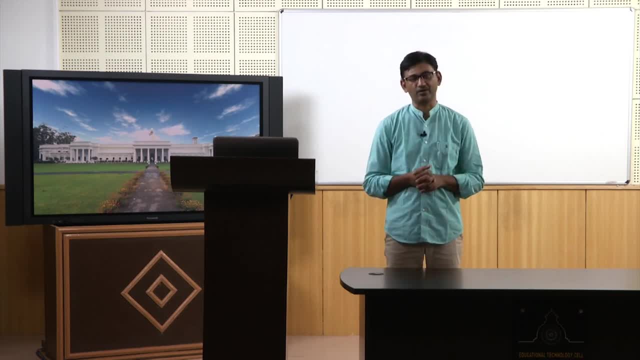 at this room temperature and pressure, for example, normal pressure. okay, That means it is not a stable means. it should change to the stable state, which is basically free carbon. okay, but it is not going to change. okay, the reason is that it is a. 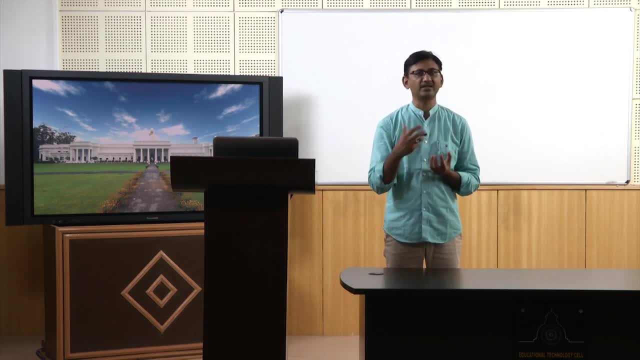 it has another condition, which is called meta stable state. okay, it is not exactly unstable, it is not exactly stable, it is in between that which is called meta stable state. okay, so diamond can exist in a condition where it is stable. 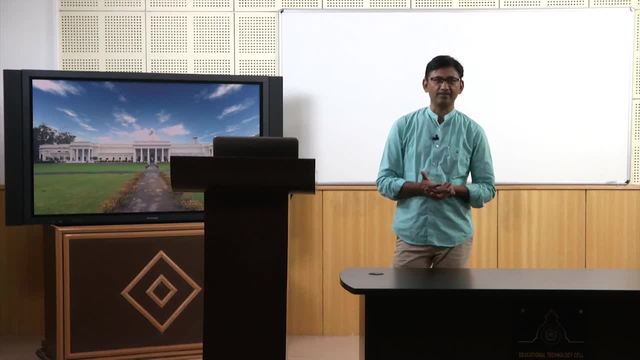 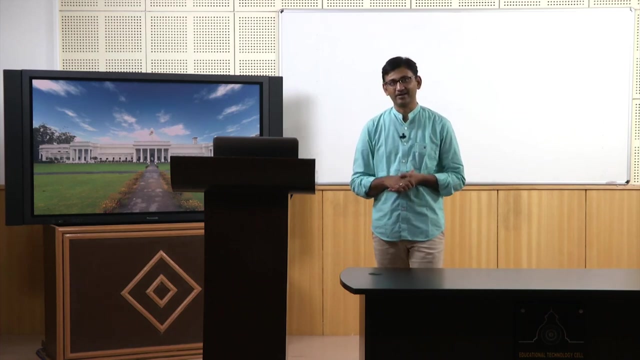 Okay. So it is not stable and you can understand people buying expensive diamonds. okay, and they must be knowing that it is going to stay like that forever. okay, that means that it is not going to change into carbon if I buy and keep it in my drawer and after few days, 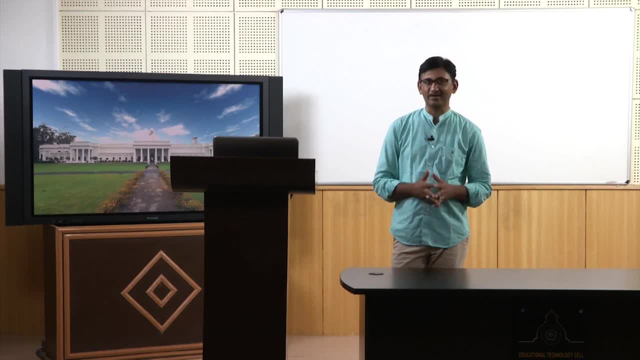 if I see that and if it is change into free carbon, then we will have a problem. okay, so it is not going to change. it is in a meta stable equilibrium. Okay, And we will see that. why it is not going to change into free carbon. okay, but before. 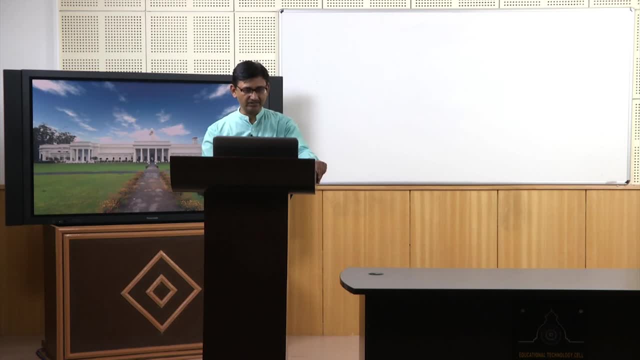 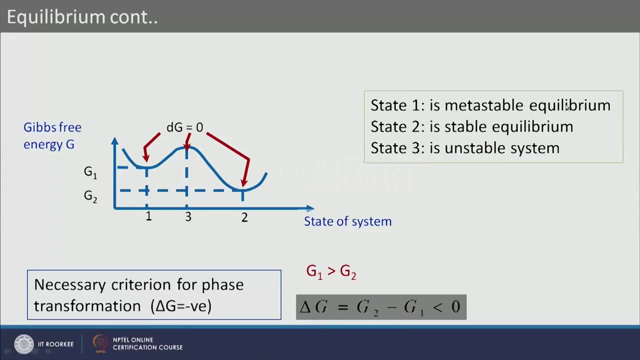 that another way to explain these 3 conditions. okay, these 3 states at which DG is equal to 0,. okay, so state 1 we are calling as meta stable equilibrium, state 2 we are calling as stable equilibrium and state 3 we are calling as unstable in unstable condition. okay, 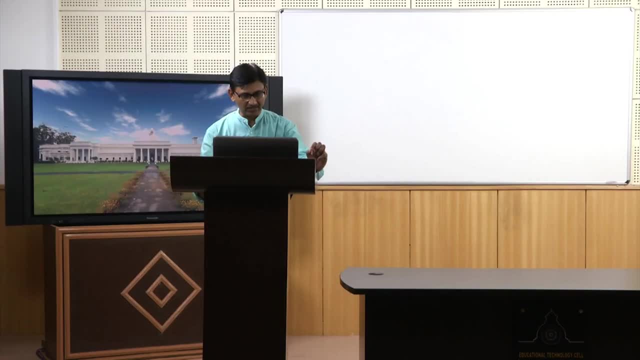 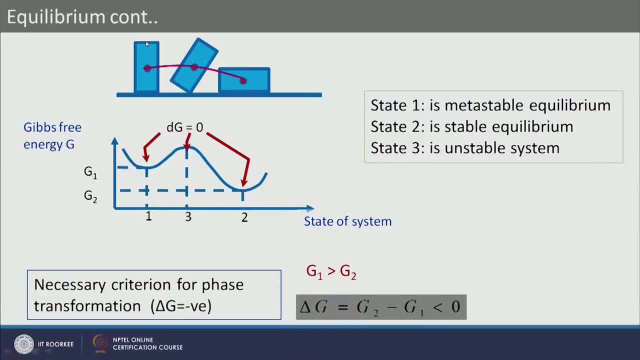 2 kind of conditions, Okay, Okay. So to sort of bring out this idea more, let me give you another analogy. okay, suppose you have a box of this shape, okay, and these points are shown, that where there is the centre, 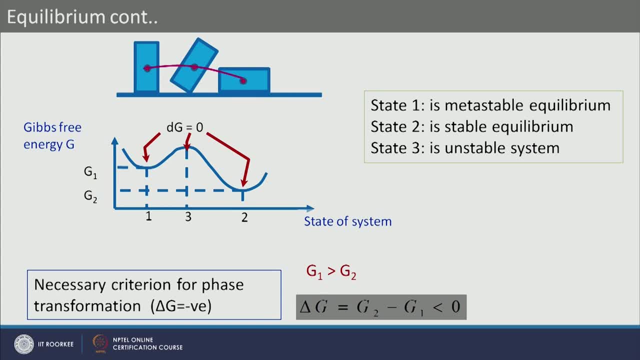 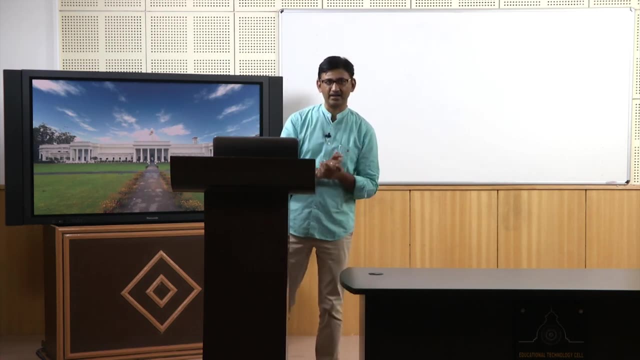 of gravity of this particular object is lying. okay, this is one state. okay, obviously, it will be more or less a stable state if I put a box like this Here, it is going to be like that. it is not going to change. okay, I can keep box in this. 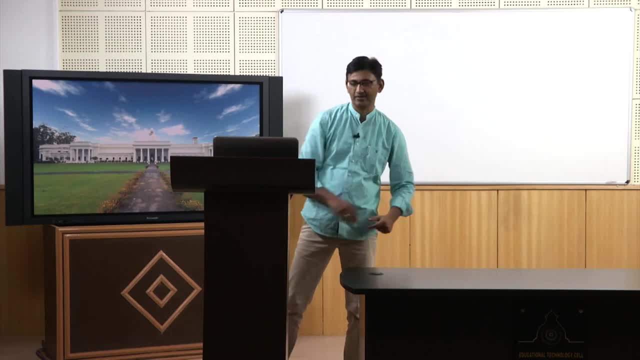 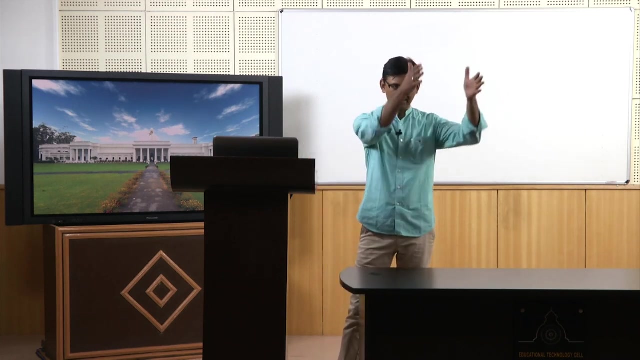 position also, so it is lying down now. okay, the centre of gravity has come down and there is another condition, which is in which I am keeping this box in a tilted condition like this. okay, now you can understand that in the first condition where I am keeping box, 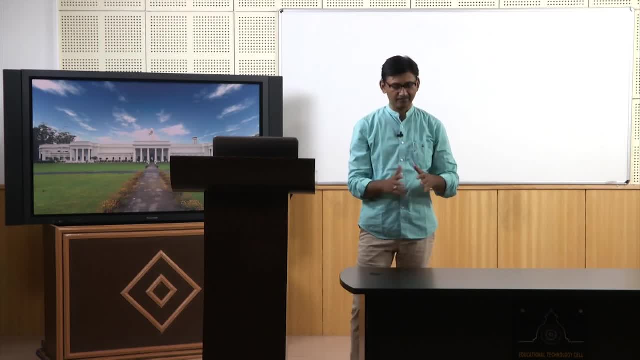 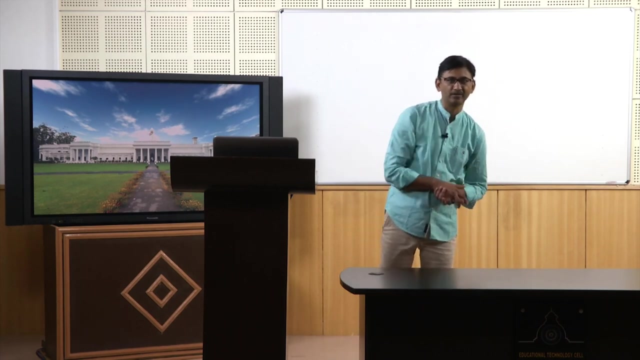 like this: okay, it will remain more or less stable. Okay, If I keep it lying down, it will be very stable condition. okay, but if I keep it in tilted on the edge, okay, either it is going to come to this position or it will go and lie down. 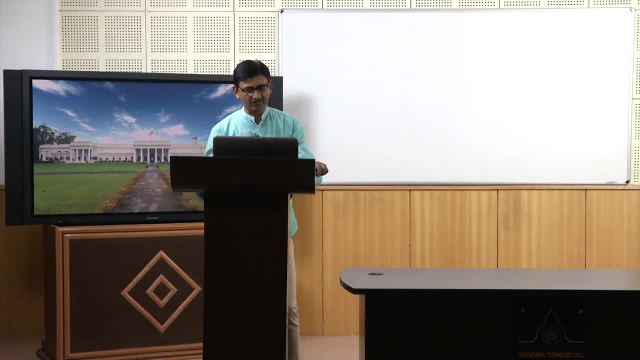 okay. so from this, if you just see, from the centre of gravity point of view, this is the most stable state for this box. okay, this is also a stable state, but it is a metastable state. Okay, If I push it, if I give a nudge, maybe it will fall down and come into this lying position. 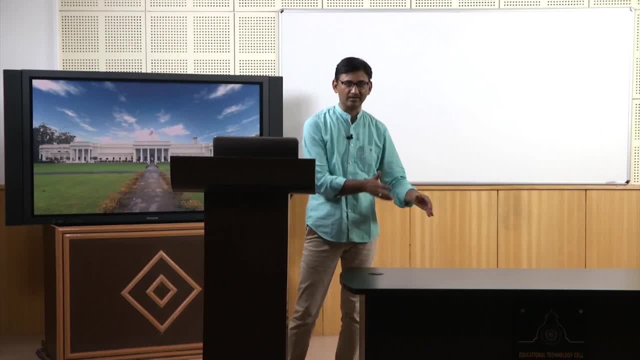 From lying position: okay, if I give it a nudge, it is not going to change. okay, so it is more stable state. okay, a small change is not going to change its status or its state, Whereas in this particular condition, the tilted condition, it is always either going. 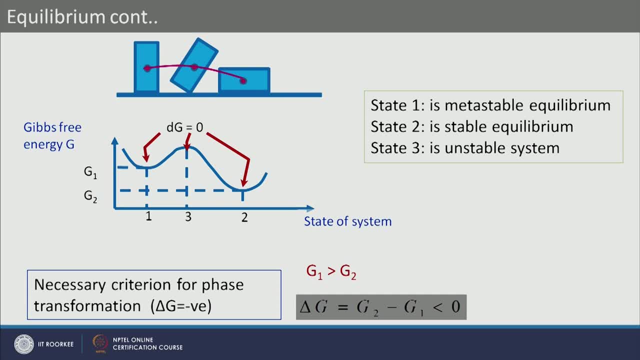 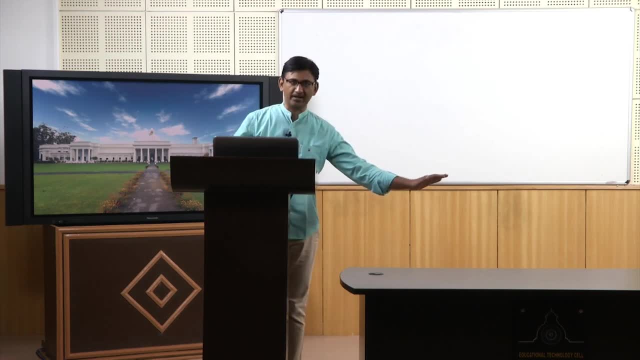 to fall in the metastable condition or a stable condition. Metastable condition can be there, okay. if I push it, maybe it will go to the lying position. or if I do not apply any external stimuli, it will remain like that, okay. so that is. 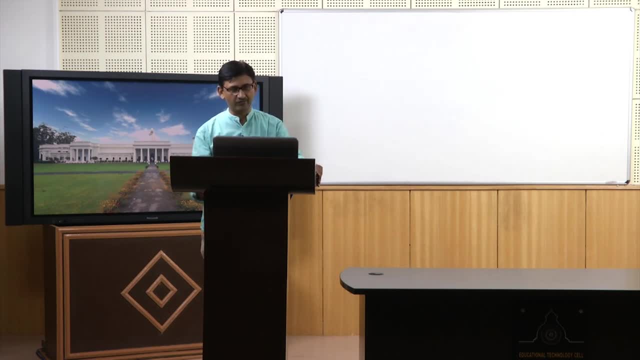 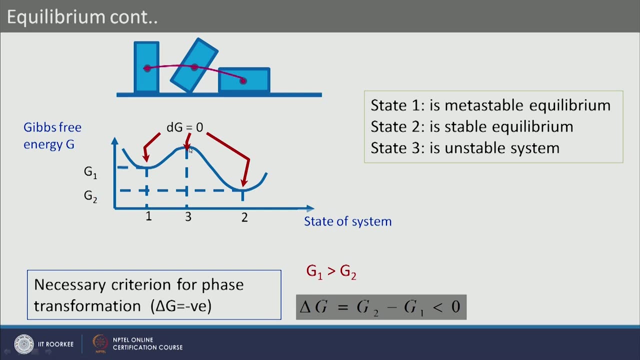 how we are defining the equilibrium here. This is the metastable equilibrium. that means it can, if any small push is given, it may like to go to the Okay Stable position, and that small push is basically this uphill which it has to cross. so it has. 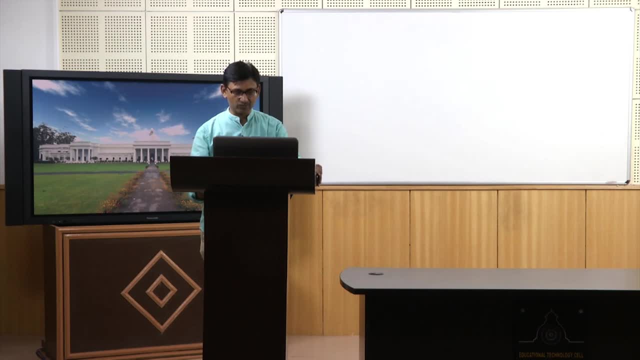 to go. the system has to go from this state to this state and then will come down to the stable state, so that much energy is required For unstable system. you do not require to do anything. any small perturbation will bring it down to either metastable state or stable state. 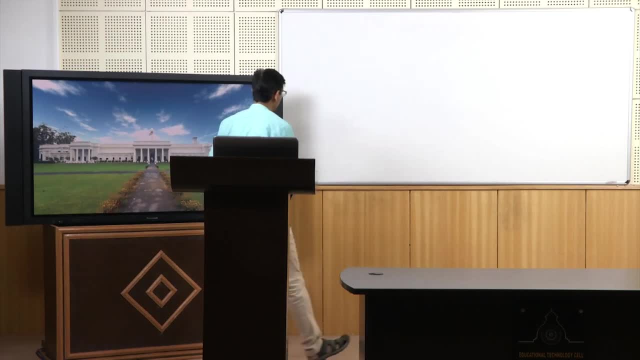 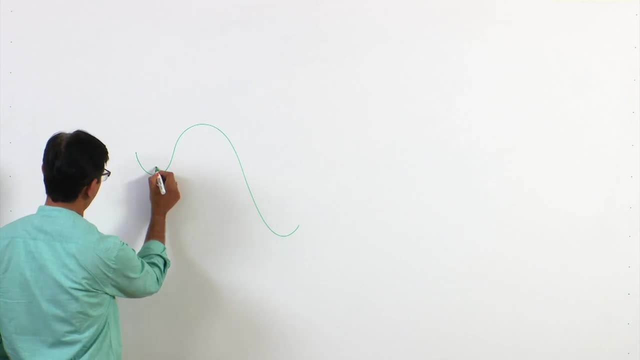 Okay, So you can think of this particular thing as a. it is like this: let us say, suppose I keep a ball here and try to take in these two direction, it will again come back to the bottom position if I keep a ball here, okay, and if I just do give a small push it. 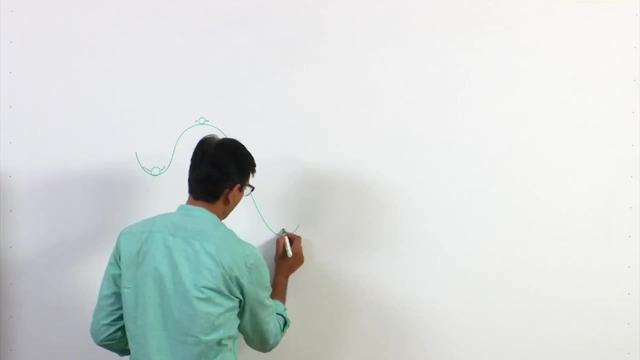 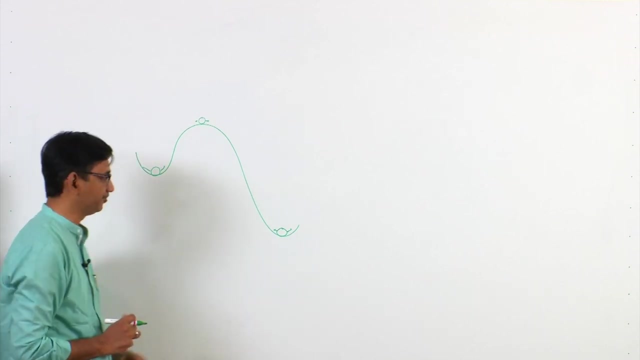 will either roll down here or roll down here, okay, and I have another ball here. In this case I am also going to. if I change the state, okay, it will try to come back to the position where it has minimum potential. okay, so, any change, you can see that it is. 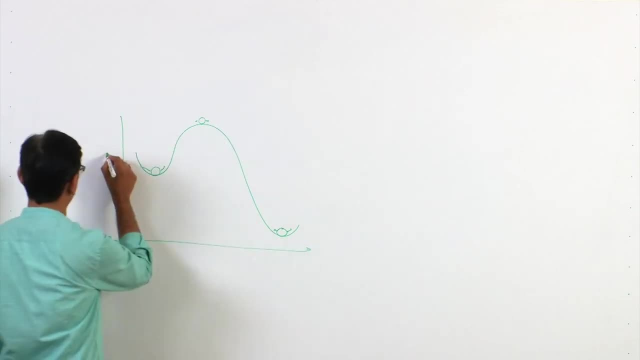 going to change the increase the free energy. okay, any change here. it is going to increase the free energy on both the side only at this position. any change is going to bring down the free energy of the system. So this is the unstable system. 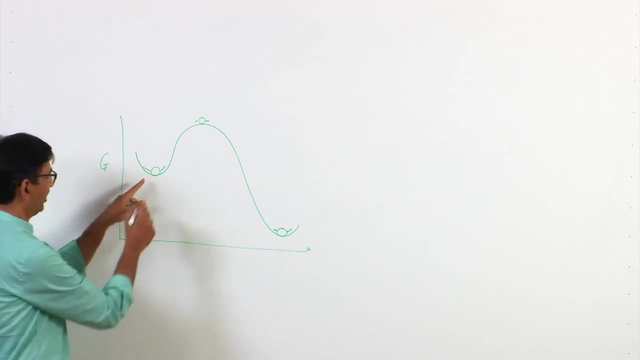 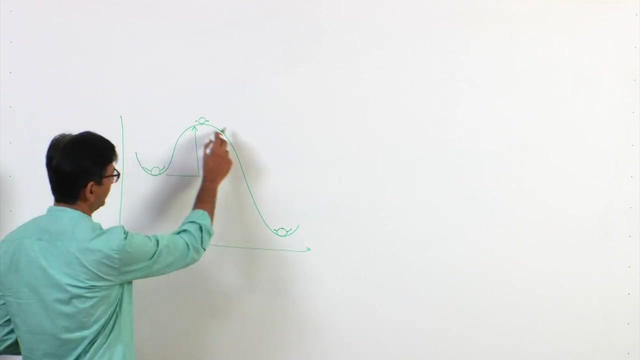 Okay, This is the unstable state, this is the metastable state. if, in from this metastable state, if I give it this much energy to the system, I will be able to bring it to unstable condition and then it will go to the stable condition. 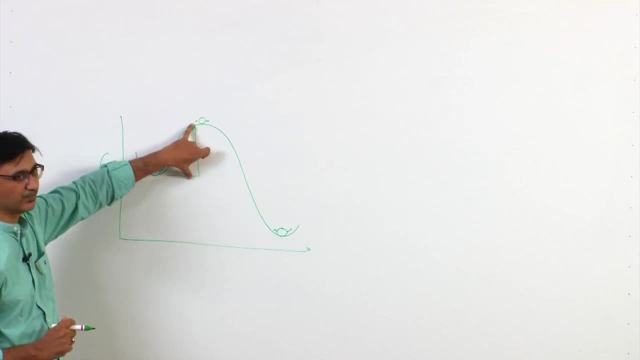 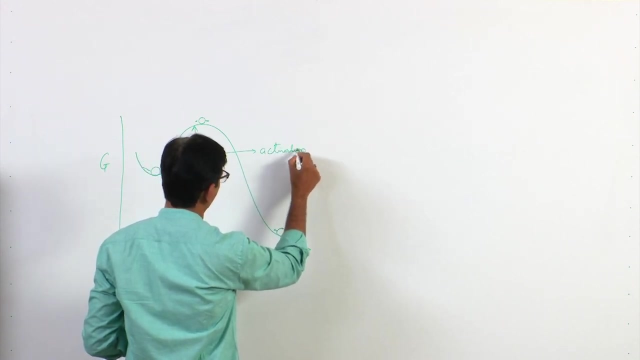 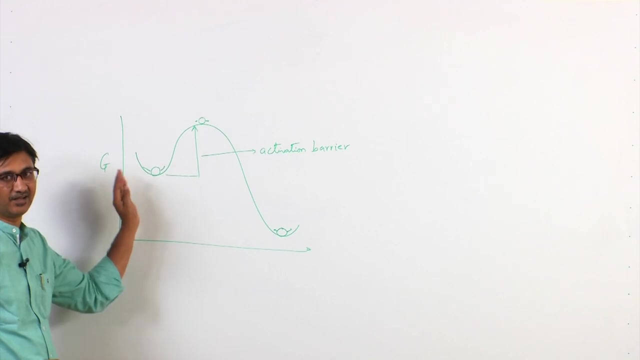 So, from metastable to stable, I need to have this much energy, and actually this is what is called activation energy. also, we saw earlier the activation barrier which has to be crossed by stable Okay, By supplying this much activation energy to bring it to the stable state. okay, so for. 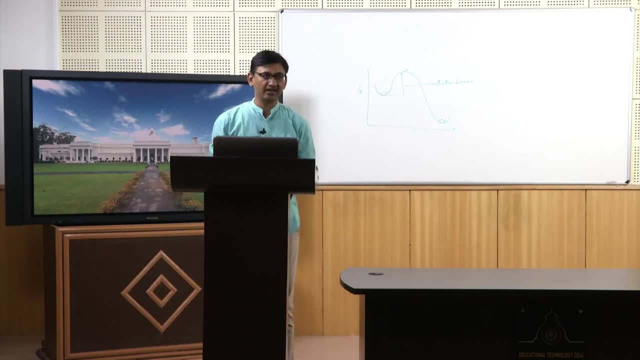 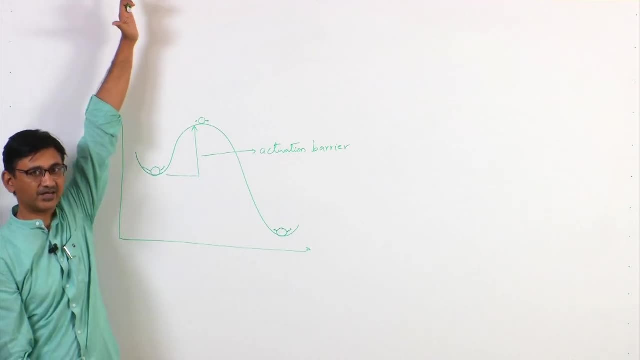 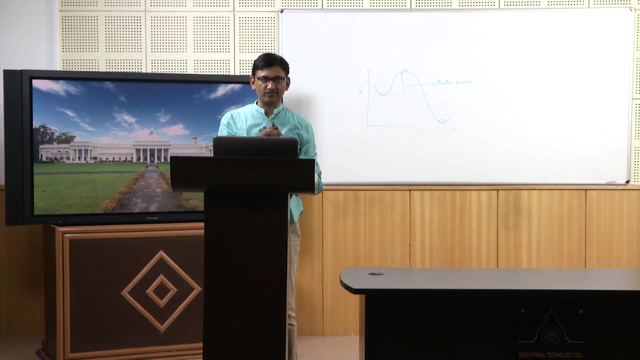 the diamond to go to the free carbon state. this activation barrier is very high. that means you require very high activation energy to take it from the state of diamond in the state of carbon, from diamond to free carbon, and that is why it is not going to change. 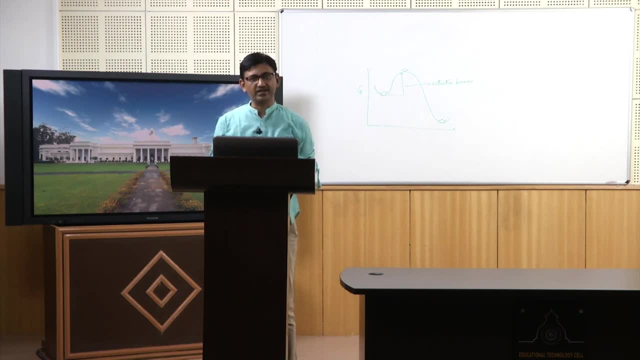 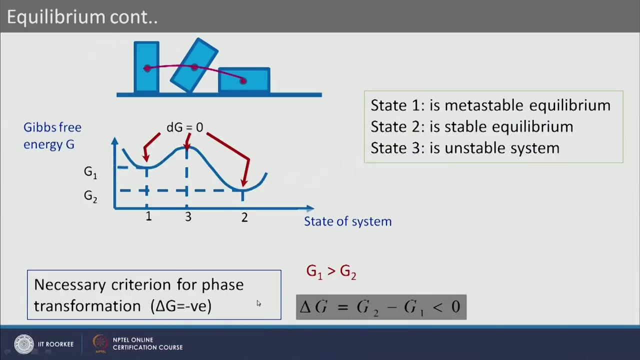 in normal pressure, Okay, At temperature condition, though it is not a stable state of carbon. okay. so that is the reason. So for any system to have phase transformation, for example, necessary criterion for phase transformation is that the change in the free energy between the two states should. 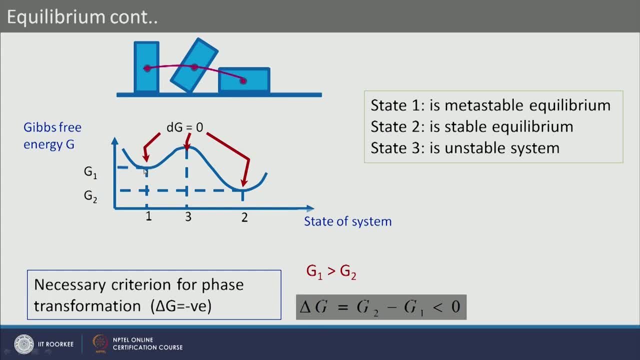 be negative. Okay, That means if I want to subtract G2 from G1, if it is less than 0, that means it is negative. then my system would like to go from this metastable condition to the stable condition. So there should be a phase transformation when this condition exists. 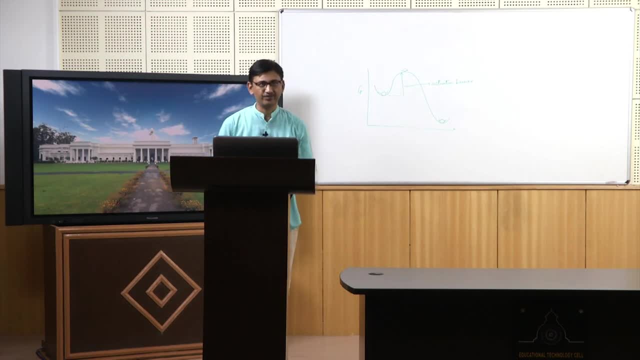 Okay, Now we will understand few terms before we go forward. Okay, For example, one term which I think you heard earlier, also when we were discussing microstructure, is called phase. Okay, So what do we mean by phase? Phase is the physically and chemically harmful. 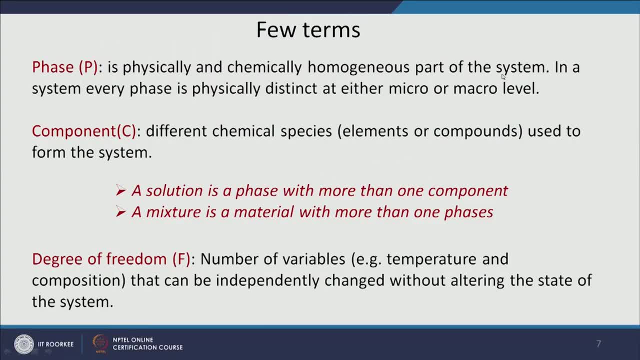 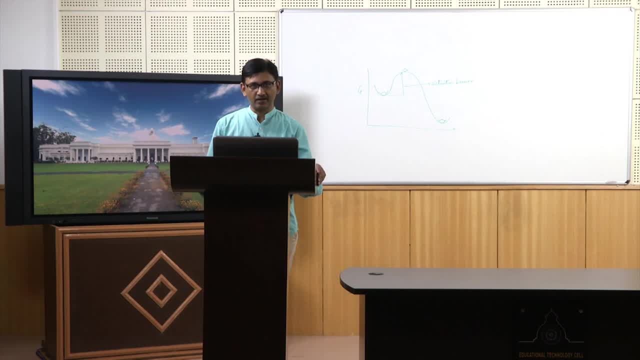 Okay, chemically homogeneous part of the system. So, for example, if I take water, it is one phase of H2O. If I put ice in that, then that is another phase. So it should be physically. in that case. chemically it is same. both are H2O, but physically it is different One. 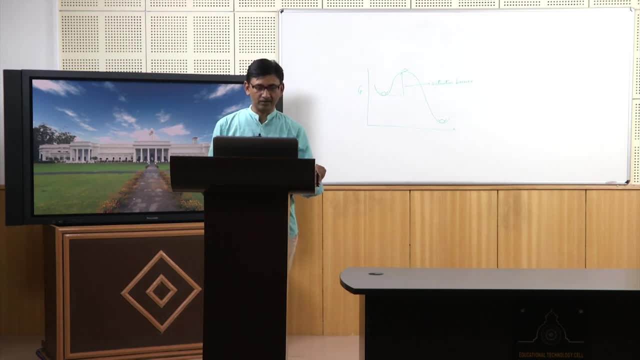 is in liquid form, another one is solid form. So when we want to call it particular phase, only water in liquid form, it is one phase. Water in solid form is ice, another phase. If I put ice in water, then these are two phases. Chemistry is same, So physically. 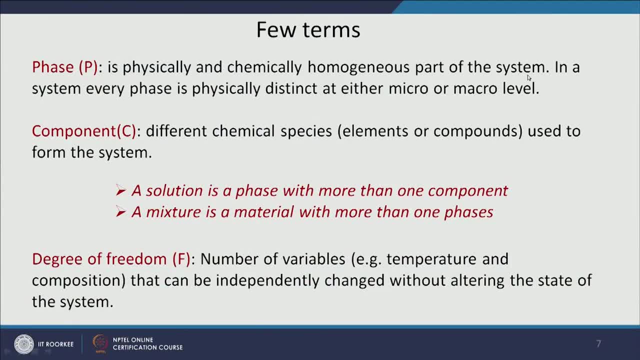 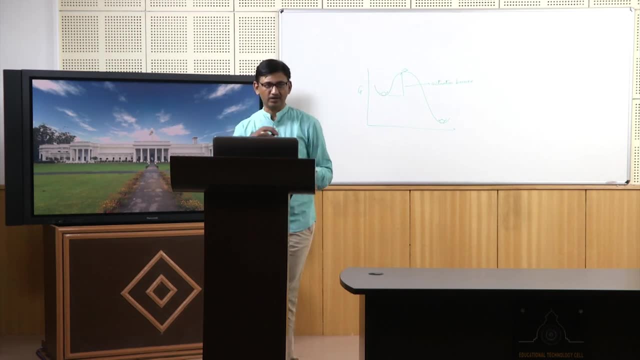 and chemically also, should be homogeneous part of the system. In a system, every phase is physically distinct At either micro or macro level. physically distinct it should be, then only we will call it as phase. For example, I can add sugar in water, So when I have just added sugar, 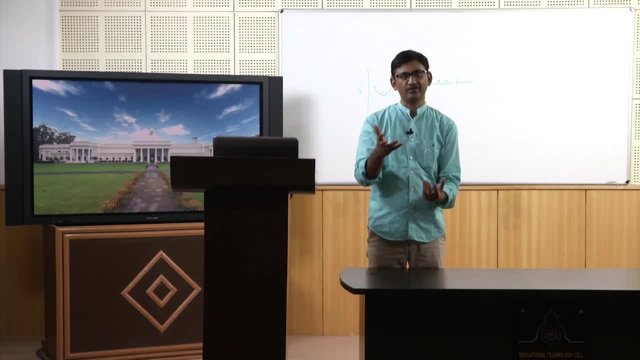 is there in solid form. water is there in liquid form. Physically they are in solid and liquid, two different forms. Chemically also it is: this is water, that is sugar, two different chemical species. So these are two phases. 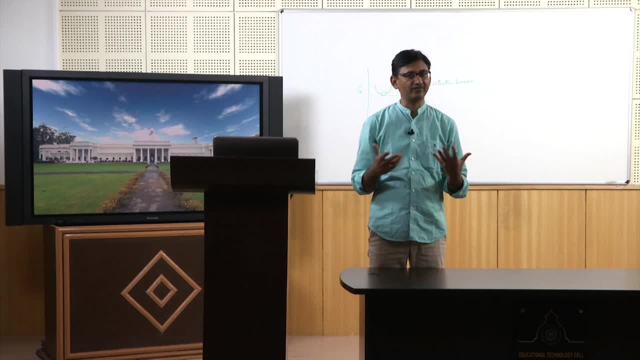 Now suppose I mix it Now after some time you will not see where the sugar has gone. So now the water is only one phase water, having sugar sugar. you can think it as a solution now, but chemically and physically it is a homogeneous mixture. I cannot see. 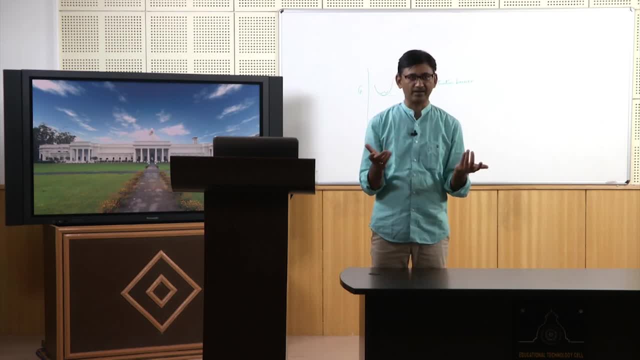 where the sugar particle has gone or where the water particle is there. So macroscopically, if I see, I do not see any difference between the two and I will see it as a homogeneous distribution of sugar in water. physically also, it will be all liquid, chemically also, if you see. 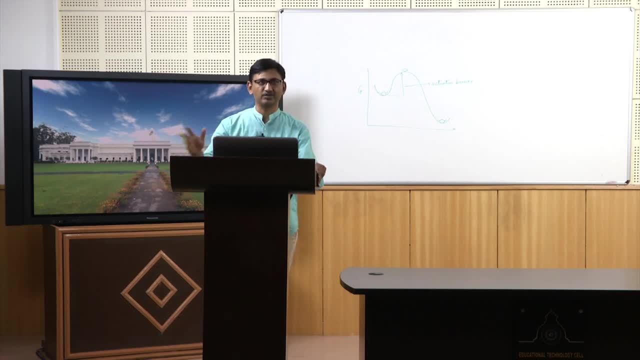 macroscopically it is going to be homogeneous, so it is one single phase. now What do you mean by component? Component means different chemical species, elements or compound used to form the system. So when I added ice into water, chemically component wise, both have one component only. 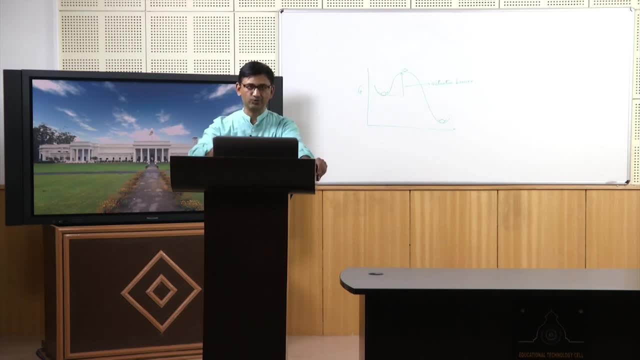 phase are two different phases. When I added sugar in water, there were two different phases. components are also one H2O, one is sugar molecule. When I mix them now there is only one phase, but still there are two components. one is 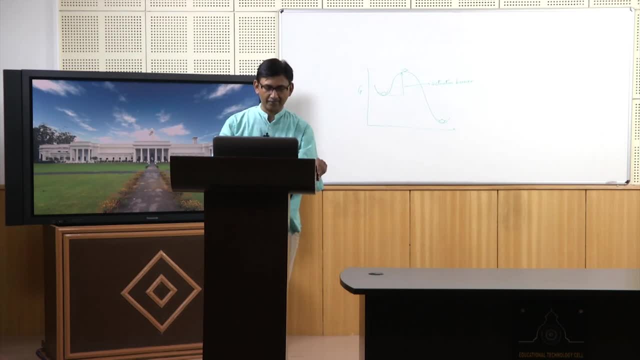 water molecule. another is sugar molecule. Okay, So a solution- if you want to understand what do we mean by solution- is a phase with more than one component. as I told you, sugar dissolved in water: it is a solution of sugar in water. 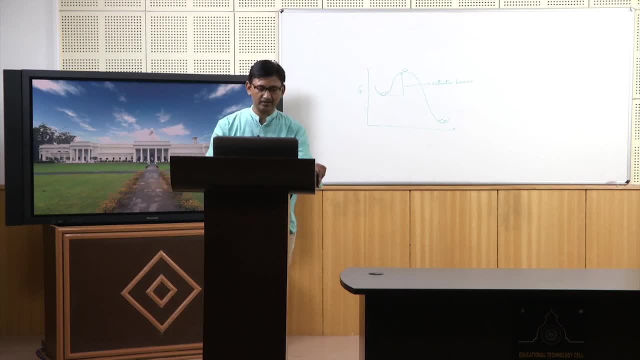 So it is a phase, single phase, but having more than one component. A mixture is a material with more than one phases. Okay, If you have two different phases, then we will call it as mixture. Okay, There is another term called degree of freedom. 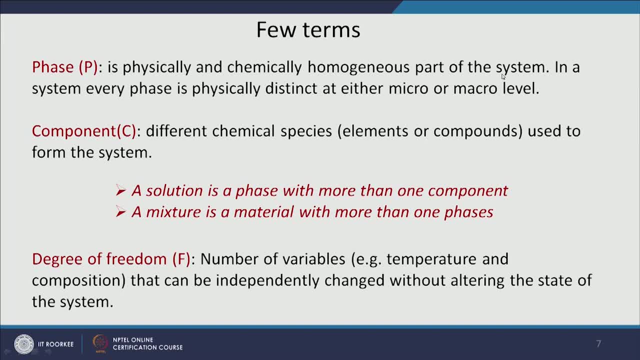 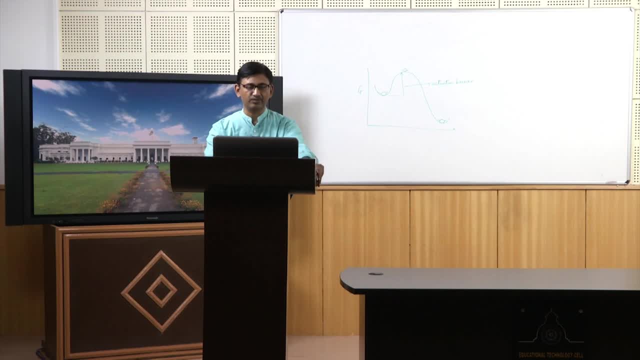 Okay, Which is basically the number of variables that can be independently changed without altering the state of the system. Okay, Variables can be temperature, composition and so on. Okay, So I can independently change them. Okay, And still I have the same state of the system. 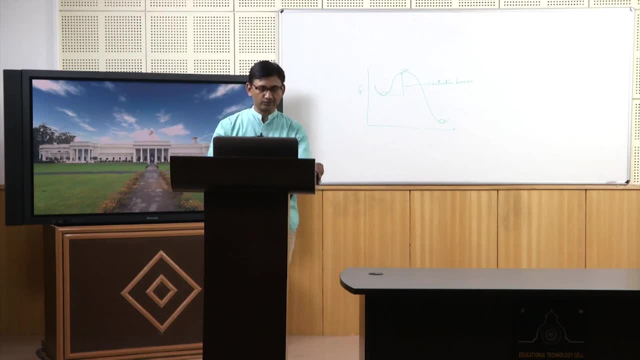 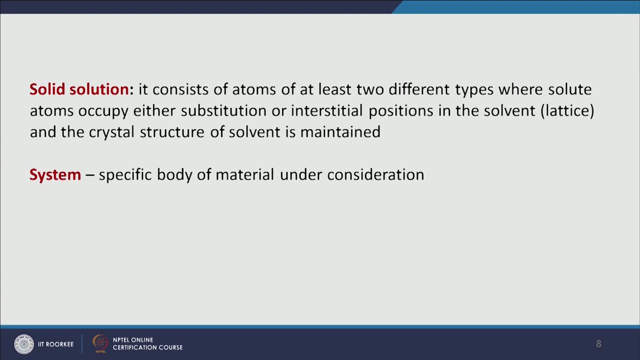 Okay. So that is the degree of freedom. I have Solid solution, Okay. Basically, it consists of atoms of at least two different type. Where solute atoms occupy ion, Okay. Atoms occupy either substitutional or interstitial positions. We have discussed this in defects, that an atom can occupy a substitutional position. 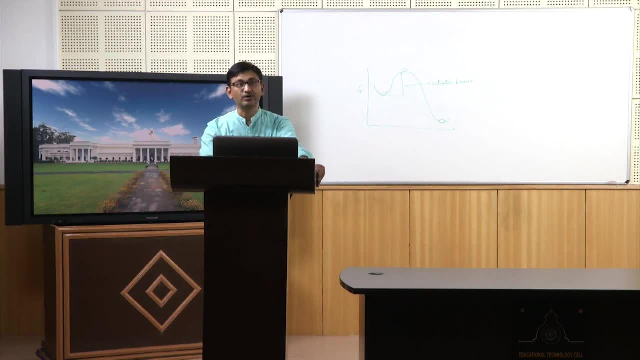 or interstitial position. Okay, So these are called solute solution, So it can be either substitutional solute solution or interstitial solute solution, depending upon the atom is occupying substitutional position or interstitial position in the solvent which is the host lattice. 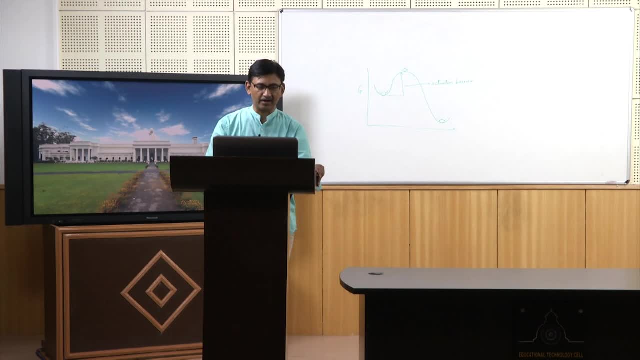 Having the solute Okay, The host atoms and the crystal structure of solvent is maintained. The most important thing here is that whatever is the crystal structure of the solvent, Okay. So when I add carbon in iron to make steel, my crystal structure of iron, which is BCC, 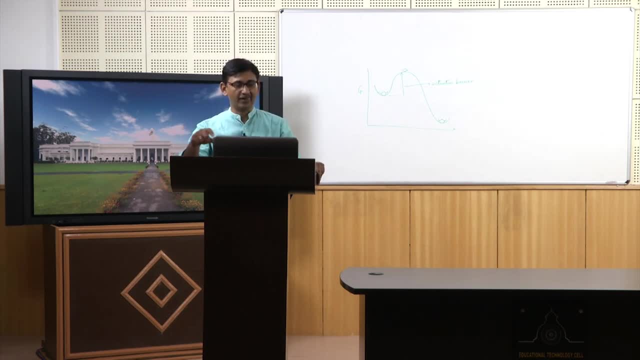 at room temperature is not going to change. Okay, So my crystal structure of solvent should not change. when I am adding any atom. Okay, Or any I am, I am adding any solute atom. A system is basically a specific body of material under consideration. 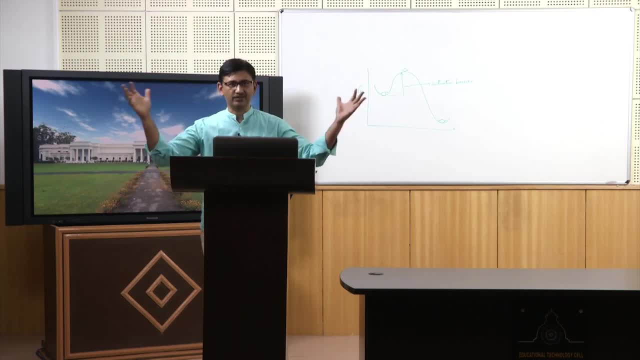 So in thermodynamics also, you must have seen that you can define system in different ways. Okay, So that is what you, the given material which you are considering, that can be called as system. Now coming to Gibbs phase rule. Okay, A very important relationship to understand the phase diagram. 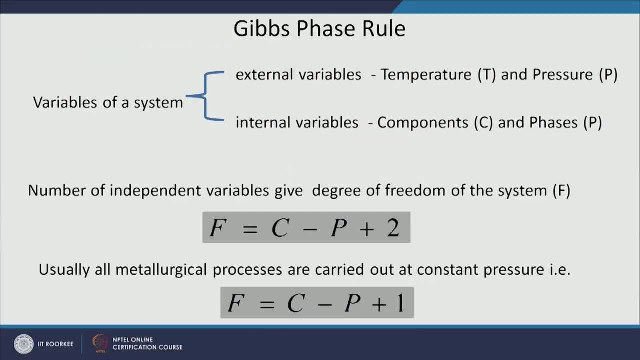 Okay, There are different type of variables of a system. Okay, Some are external variable, like temperature and pressure, Some are internal variables, like components and phases. So the number of independent Gibbs, free Gibbs, phase rule actually gives the relationship between the degree of freedom a system has and the variables which are there in a system. 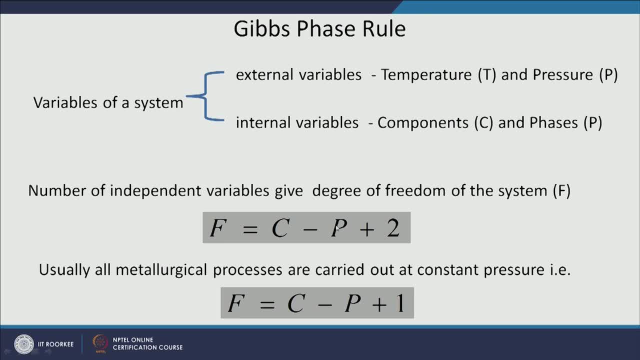 So component C will be one variable, Phase will be one variable And there is one constant element. Okay, Okay, And added 2 here, that is to take care of temperature and pressure. Okay, So plus 2 means one is for temperature, one is for pressure. 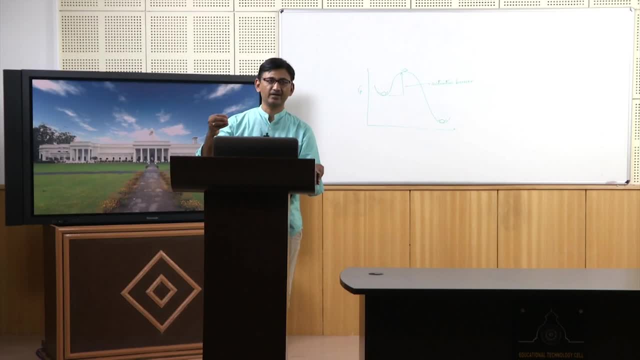 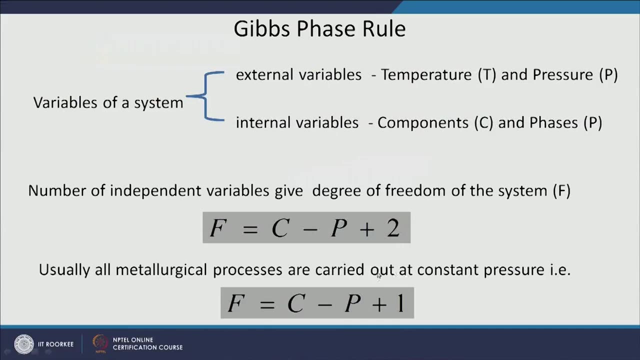 So how many variables are there? Okay, That will give me independent variable, that will give me the degree of freedom a system have. So usually, because all metallurgical process are carried out at constant pressure, because we do not change whatever is the normal atmospheric pressure is there, in that we do all the heat. 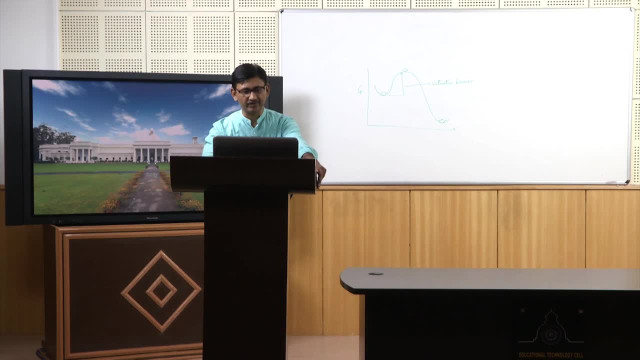 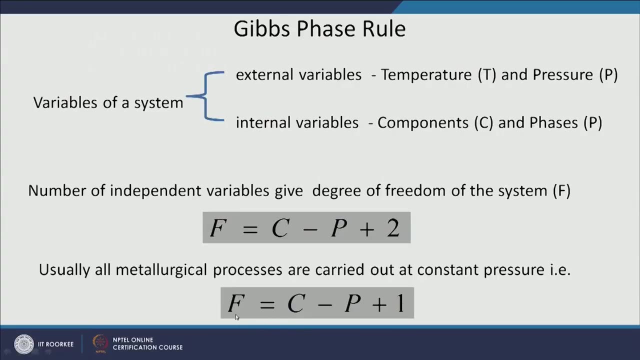 treatment or solidification or melting or whatever. Okay, We will take out the pressure from this equation. So now, instead of 2, we will only have 1 here. So now my degree of freedom will be calculated from what is the number of components in the 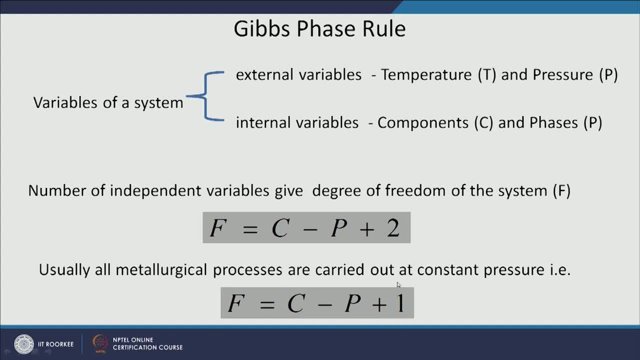 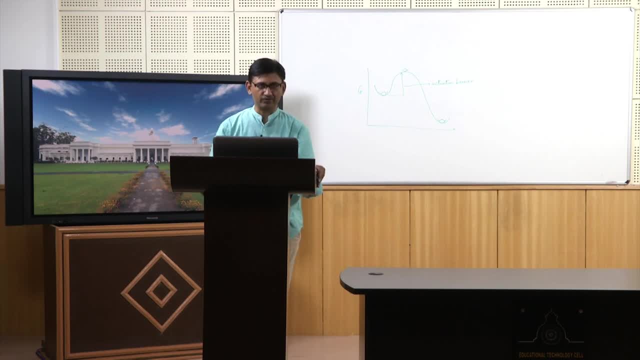 system. What are the number of phases in the system? and 1 for the temperature? Okay, So this is the Gibbs phase rule. I have not gone into the derivation of that, but we do not have to worry about that right now. Now, 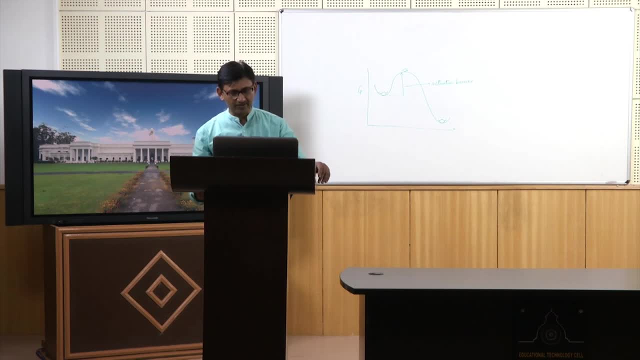 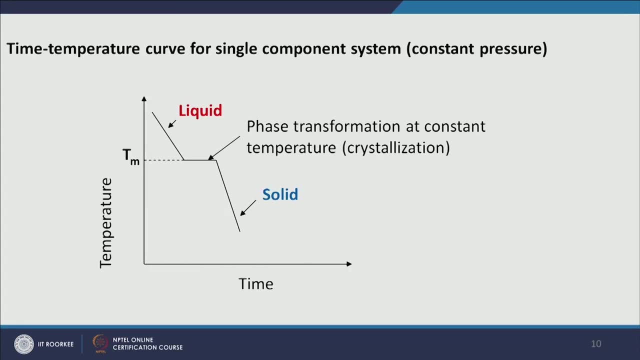 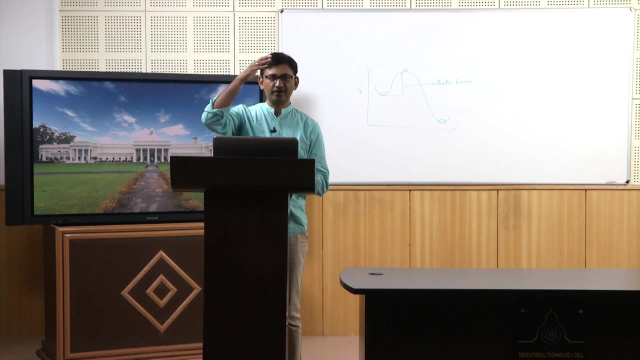 Okay, Let me just use this particular Gibbs phase rule in one particular condition, for example. the second one is a. this slide shows you a time temperature curve for single component system. That means, if I do solidification, or let us take water from liquid state, it is going into. 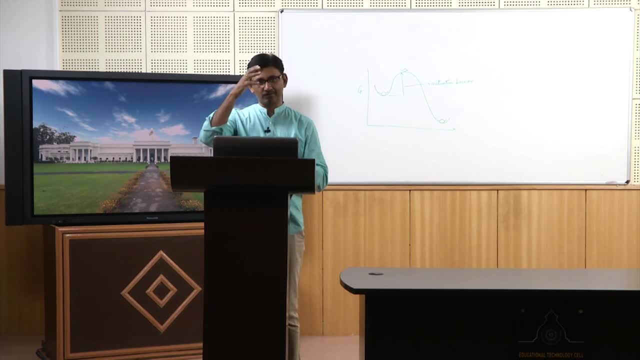 solid state. Okay, So we have taken water. we are continuously decreasing the temperature of the system. Okay, By some external means, and we are measuring that, how the temperature is varying. Okay, We have put a thermocouple there, So temperature is coming down in the liquid state. 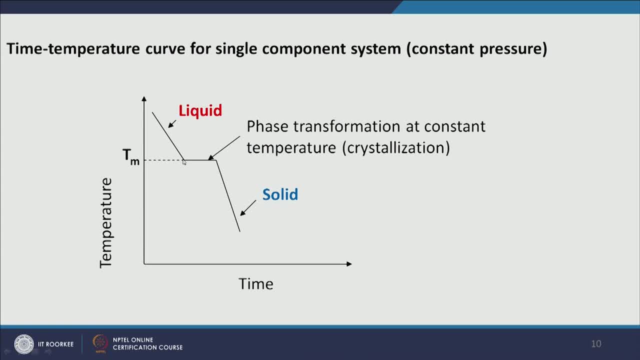 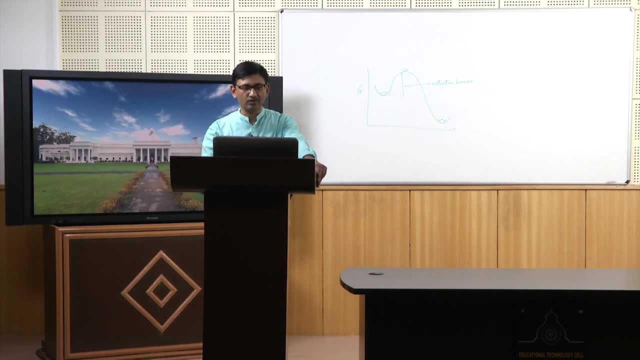 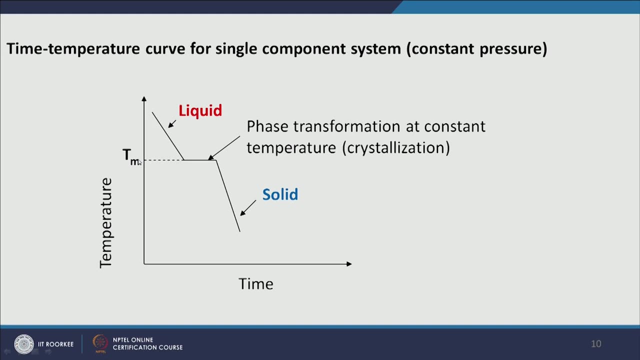 Okay, At some point where the transformation starts from liquid to solid. Okay, That we know that The whole phase, transformation from liquid to solid, will happen at a constant temperature, which is we can call as melting point, Okay, Or solidification point. 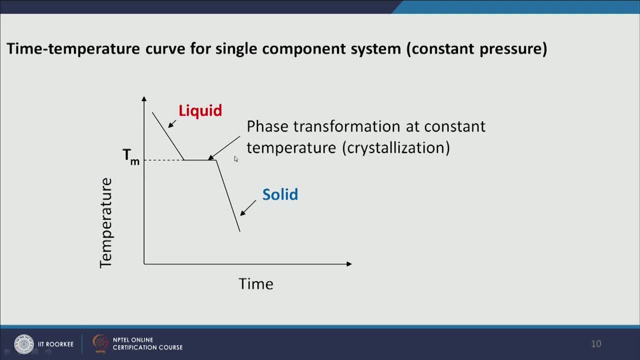 So we are. we are saying that it is TEM. Okay, So phase transformation is constant, temperature is happening here, crystallization and after complete solidification, now the temperature is coming down in the solid. Okay, Now, this is a one component system. We have taken one liquid, let us say water, pure water. 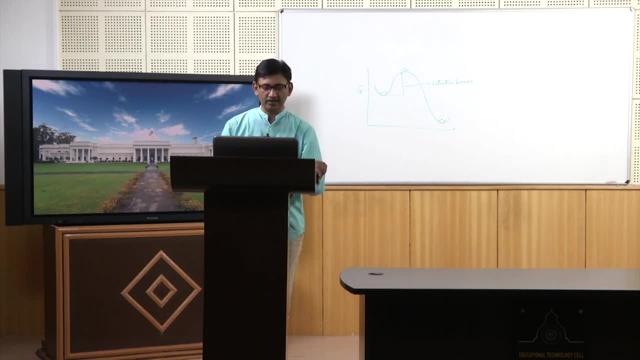 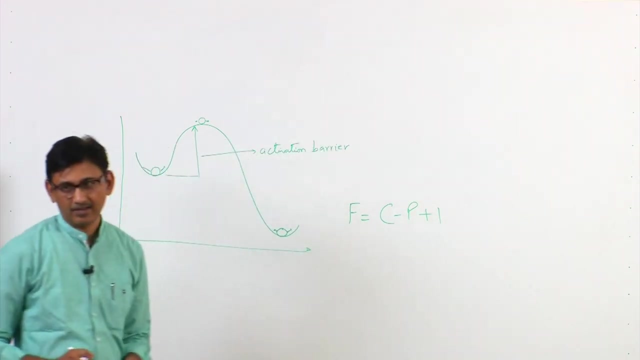 Okay, And for that we have done this experiment. Okay, When it was a liquid, If you apply Gibbs-Freyers rule, which was, if you remember, F equal to C minus P plus 1.. Okay, Now when, what is? when it was in liquid state? 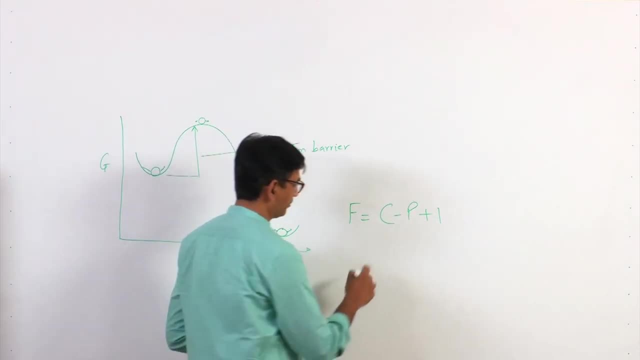 Okay, You had one phase, one liquid phase. You had one component, which is the water. Okay, So 1 minus 1 plus 1 will give you F equal to 1.. Okay, So there was one degree of freedom, Okay. 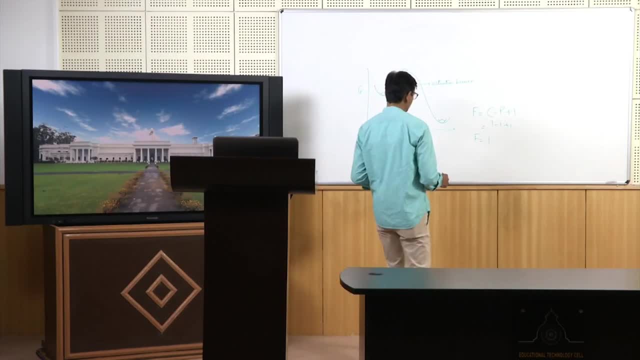 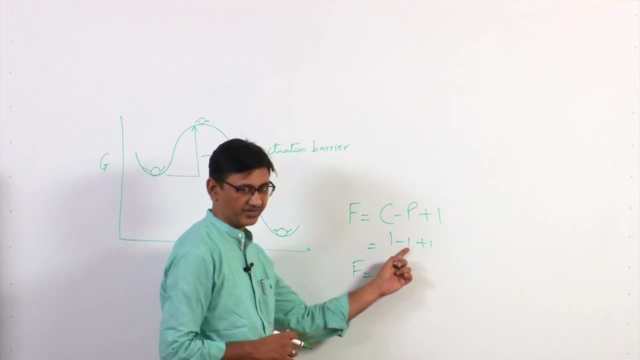 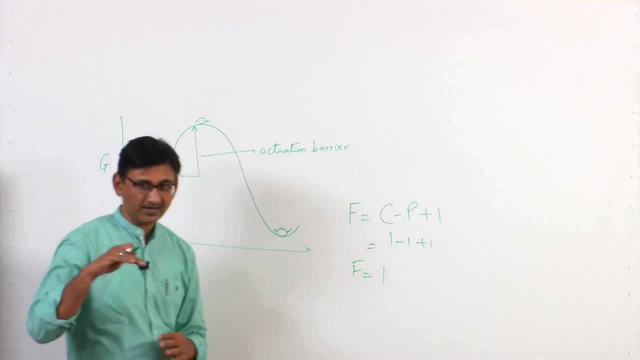 When it was in liquid state, When it was in solid state. again, you can do the same analysis. It is one solid one water molecule, one phase, that is solid phase plus 1. again, you will get the degree of freedom as 1.. What happens? 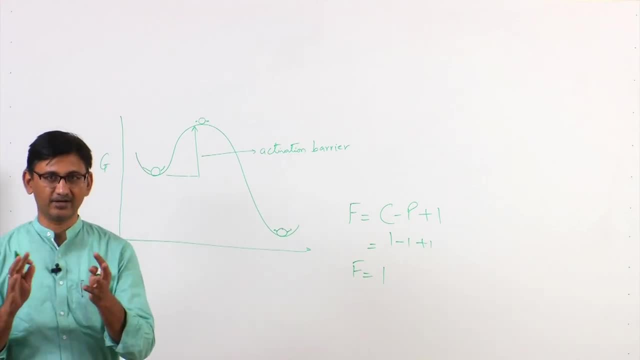 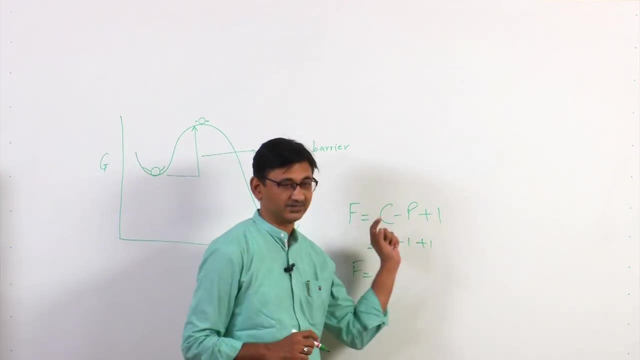 It is doing the transformation. Okay, So we know that at the transformation the solid and liquid are in equilibrium. Okay, That means now you have two phases. So if I again do the same analysis for degree of freedom, component is same. it is all water. 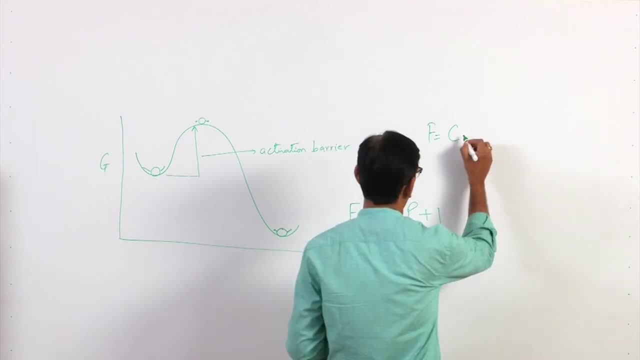 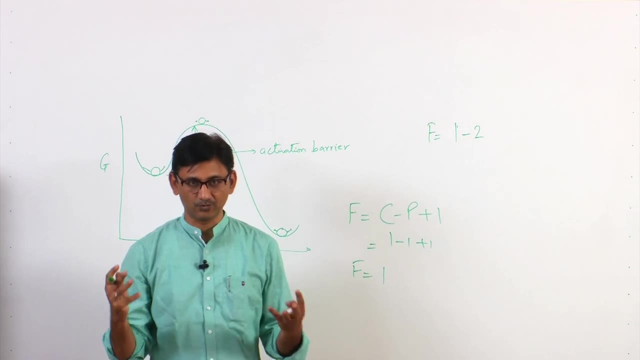 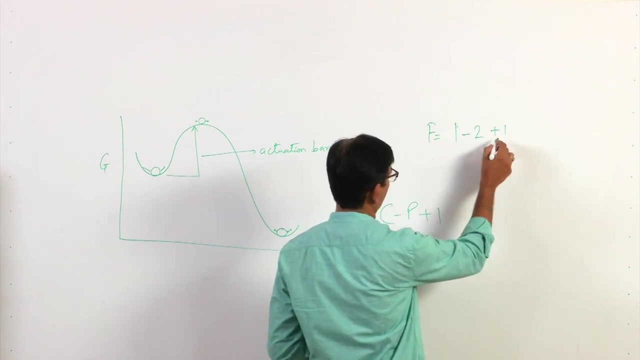 whether it is in solid phase or liquid phase. Phase, you have two. Sorry, I will write 1.. Okay, Because it is two phases in equilibrium. Okay, And plus 1.. This is 1 minus 2 will be minus 1. minus 1 plus 1 will be 0.. 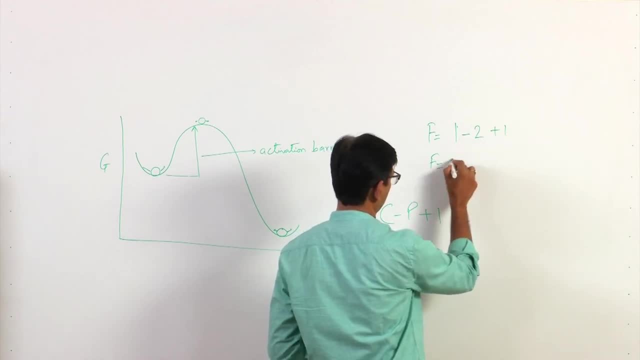 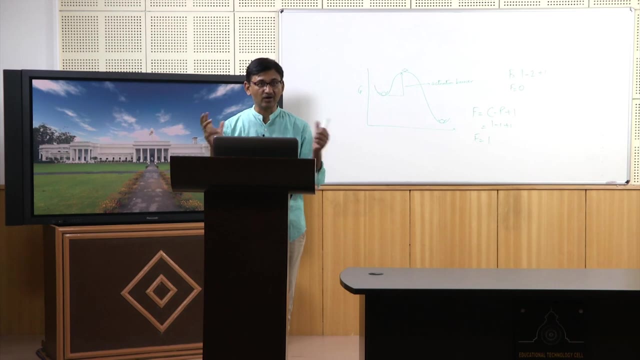 So this is, the degree of freedom is 0.. So now you understand that because degree of freedom is 0, that is why the transformation is happening at a constant temperature. I cannot change the temperature now, So for this particular case, when the transformation is taking place, it is going to take place. 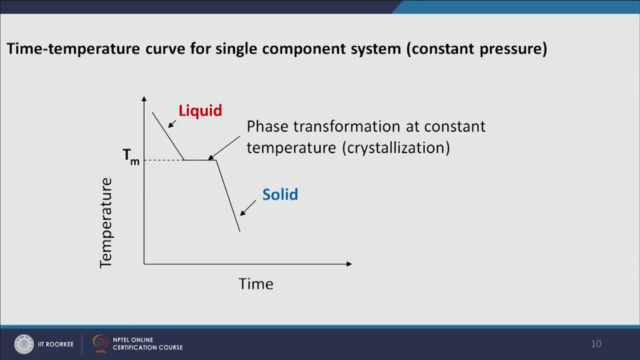 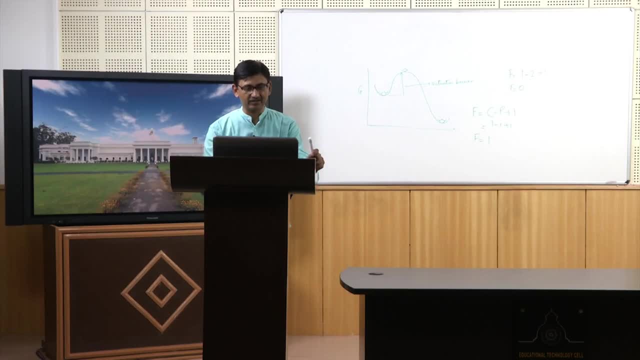 at a constant temperature. Okay, So my degree of freedom of the system is 0. I cannot change anything. There are no independent variables. All the variables are fixed, Okay, And that is why the temperature is also fixed, and I cannot have any variation in the temperature. 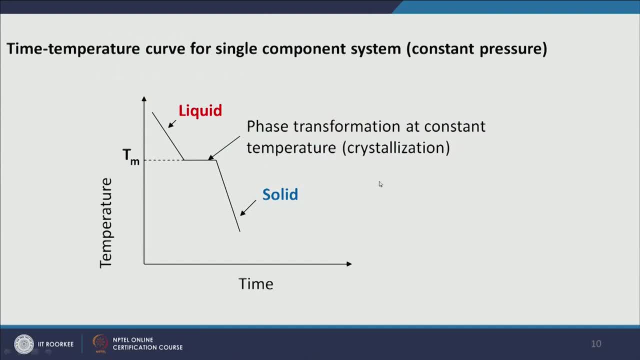 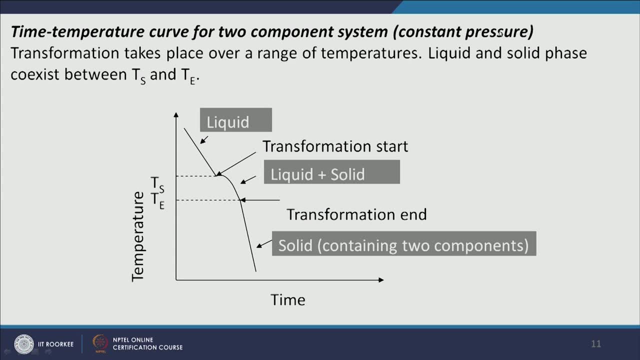 The transformation has to take place as constant temperature- Okay, This is another case time. temperature curve for two component system- Okay, At a constant pressure. again, I can use the same equation. So transformation takes place over a range of temperature. Liquid and solid phase coexist between Ts and Te. 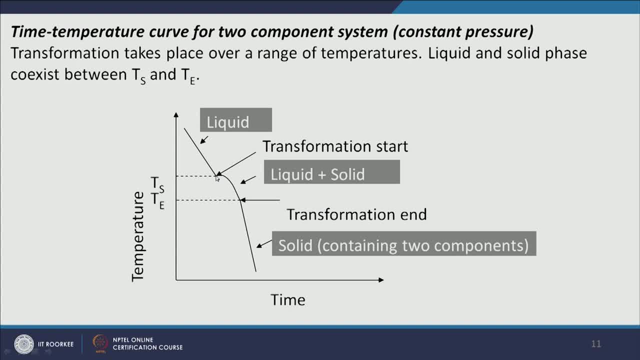 Okay, Now you see, in comparison to the previous slide, here the transformation is taking place at a over a temperature range. Okay, In the previous case, the transformation took place at a constant temperature. Okay, Why that is so? So, if you see, this is a two component system. 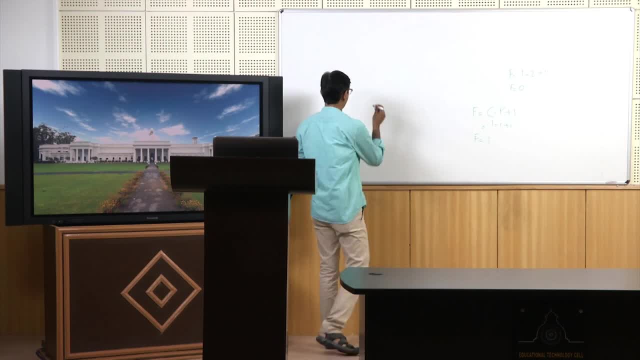 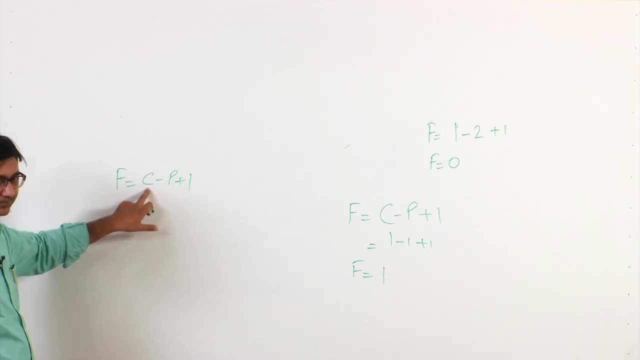 Okay, This is a two component system. Again, I can use the same equation: F is equal to C. Okay, C minus P plus 1. Okay, So components are two. where the transformation is taking place, two phases are in equilibrium, Okay. 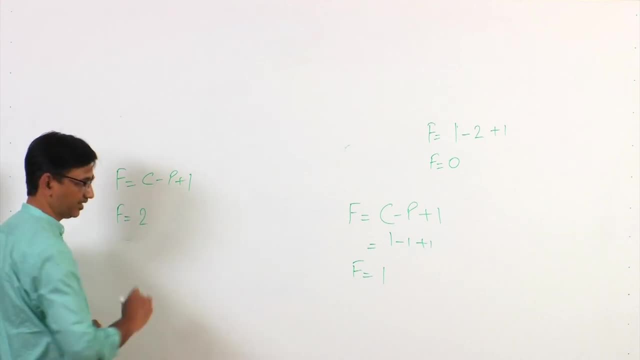 So now, if I put, two components are there. this is my two component system. two phases are in equilibrium when the phase transformation is taking place and one these two cancel. So you have degree of freedom is 1.. So now, as opposed to the previous one, 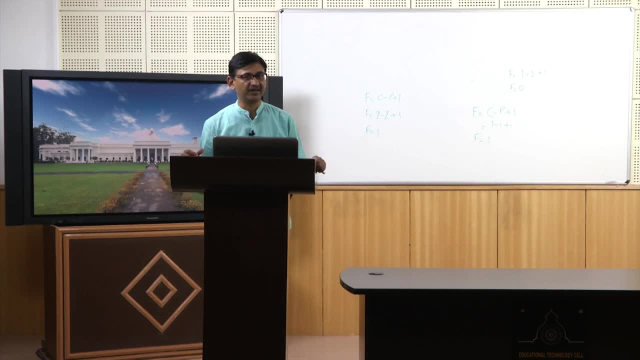 So the previous one case. I have one degree of freedom left in the system, and that is why the transformation is taking place over a temperature range, whereas in single component system the transformation from liquid to solid was taking place at a constant temperature. Okay, So this is how the time temperature curve vary between single component to component.